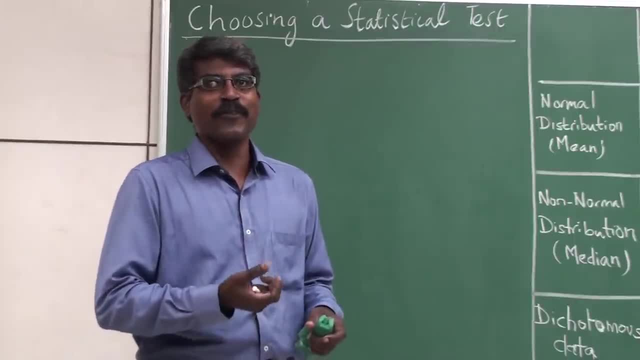 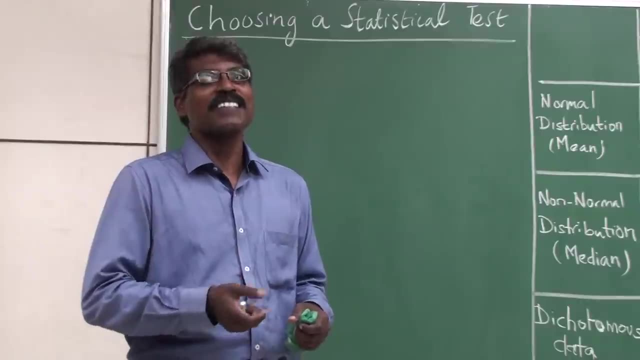 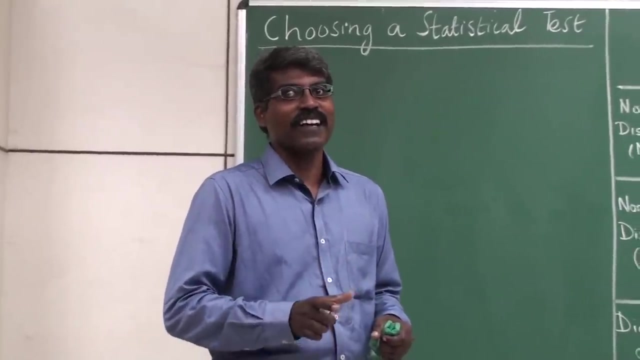 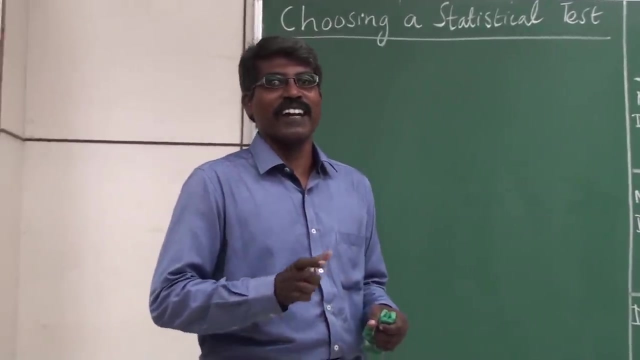 Yes, if he does not know which tool among the four he has to use now, he will tell that I will use the most appropriate tool. Same way, whenever you write the most appropriate statistical test will be used for analysis of data, then it clearly means only one thing: that you don't have any idea about which statistical test to be used for this analysis of data. 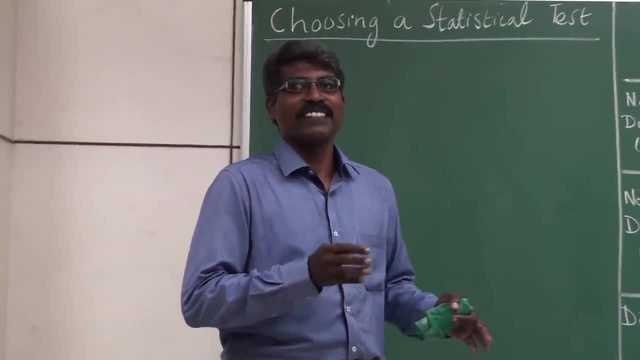 So henceforth, please don't write. the data will be analyzed. Yes, if he does not know which tool among the four he has to use now, he will tell that I will use the most appropriate tool. So henceforth, please don't write. the data will be analyzed by most appropriate statistical test. 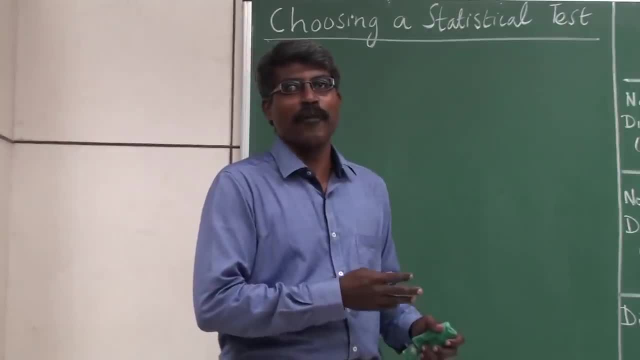 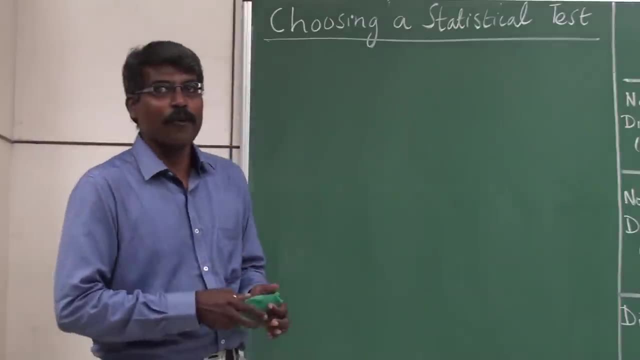 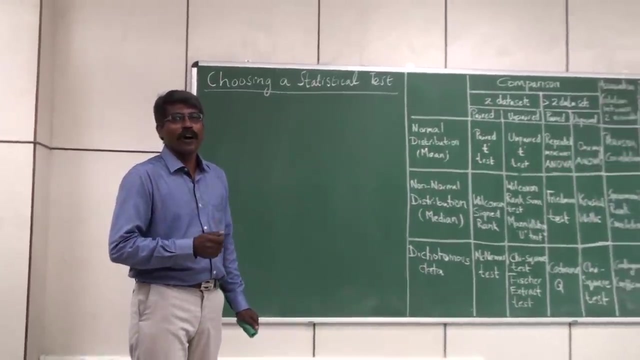 So this session will make you to find out which test you will do, so that you will not be able to write like this. Let's go into this session first. Now let's see what are the factors which determine this analysis, so that we will be able to approach it properly. 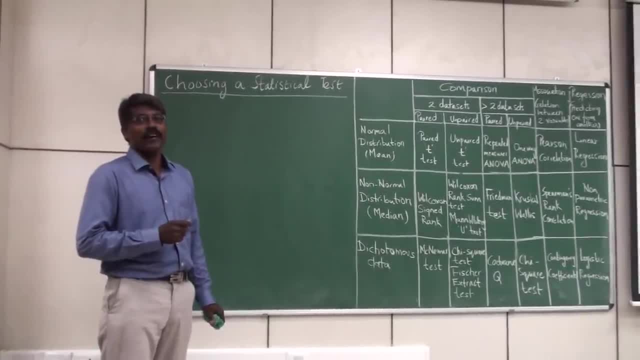 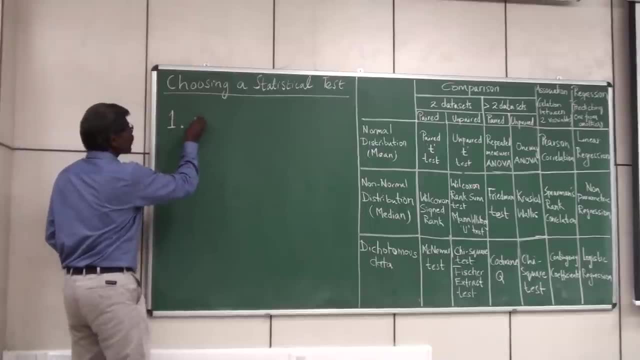 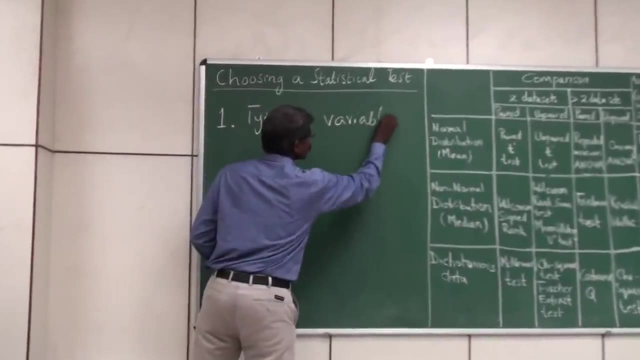 There are five factors which determine the analysis of choosing a statistical test for analysis of data. There are five factors which determine the analysis of choosing a statistical test for analysis of data, of data. Let's see one by one. The first factor is the type of variable. We have already seen. 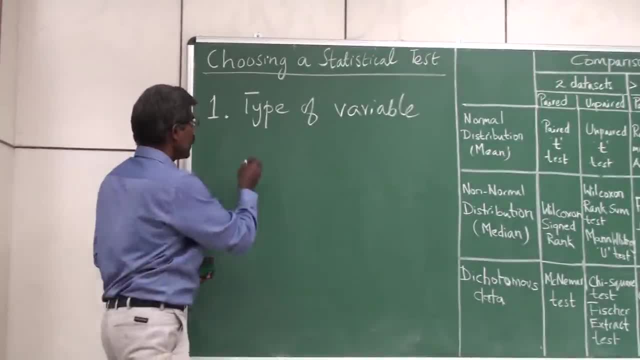 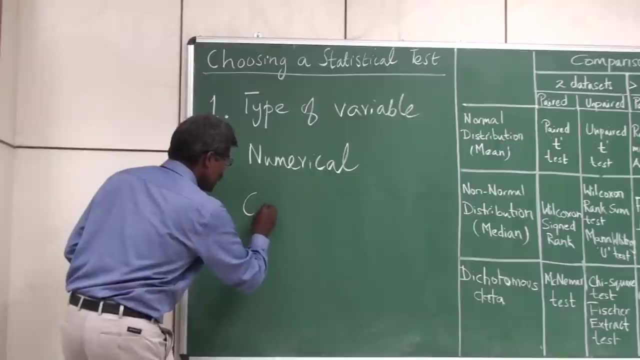 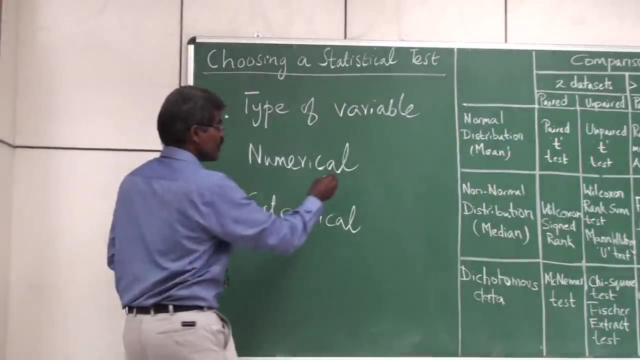 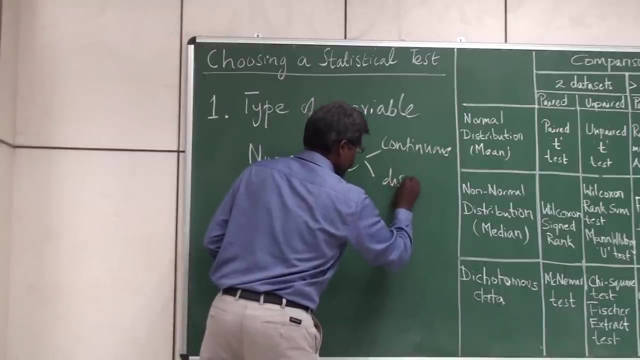 that data can be of two types, isn't it? The first one? we have seen it as numerical. and the second type of data- we have already seen it can be categorical, isn't it? Now? numerical again can be, it can be continuous or it can be discrete. One example for a continuous: 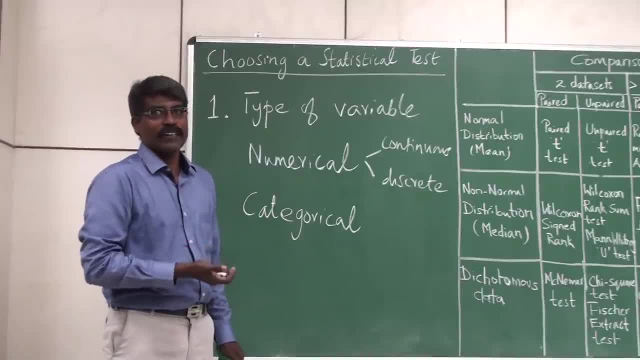 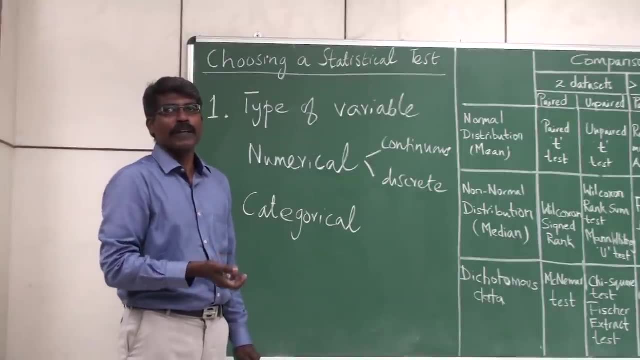 numerical: variable blood pressure, body weight. For numerical discrete we will use number of people visiting OPD or visual analog scale measured in a scale of 0 to 100.. Again, it's a numeric, but discrete Because it does not take any decimal points. Categorical: we have already seen a classical. 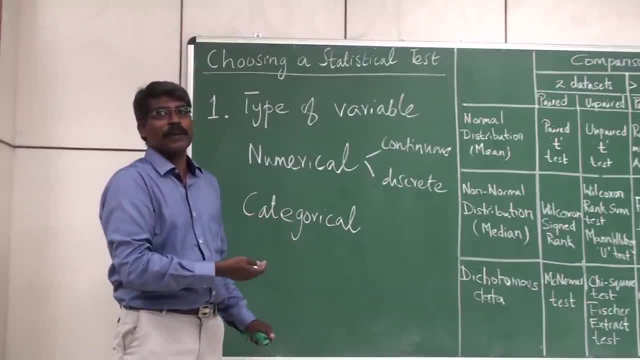 example of a dichotomous outcome. whether adverse effect, the patient experienced adverse effect or didn't experience. The patient got Q, not Q. So these are all some types of categorical data. So first we need to find out our data is numerical continuous or numerical discrete. 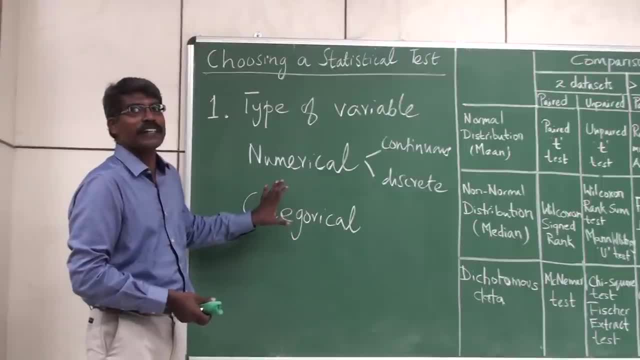 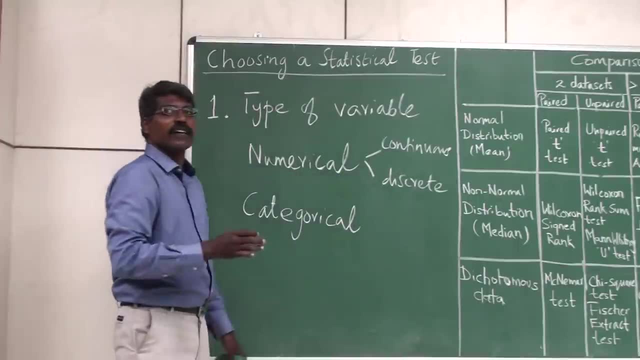 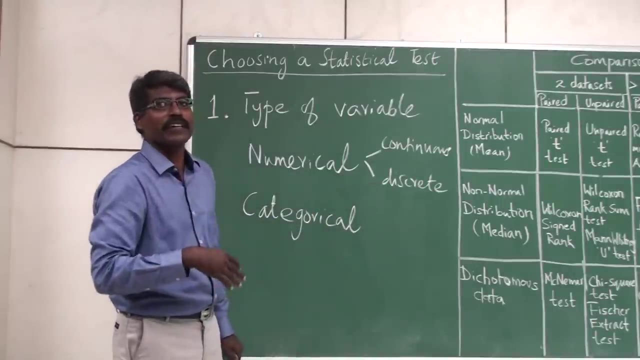 and or is it categorical? So that's the first factor which affects One more point which we need to remember. The second factor this time is if it is a numerical continuous data, it is usually summarized as means. If it is a numerical discrete data, many times it does not follow normal distribution. 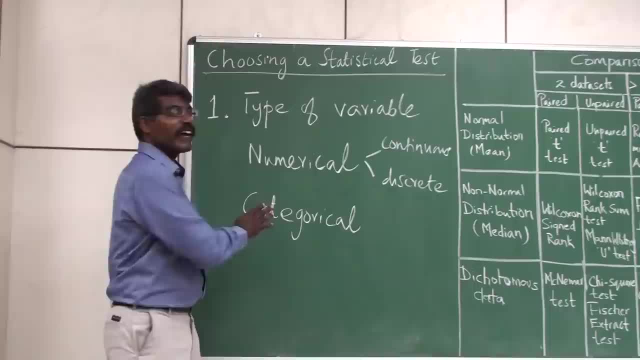 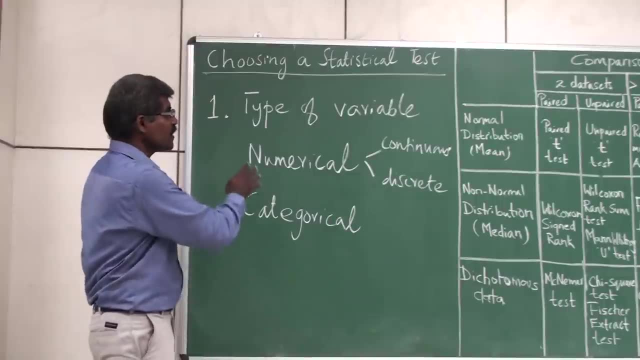 and it is summarized as medians. Categorical data are usually summarized as proportions, So we will just keep this knowledge in mind and see how it is of help. So the first thing you need to know: what type of variable do we have? right Now let's look into the second. 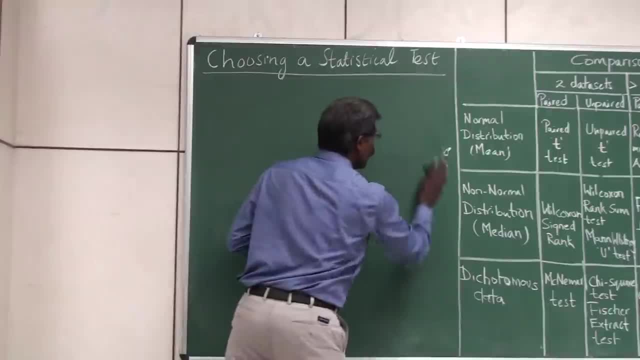 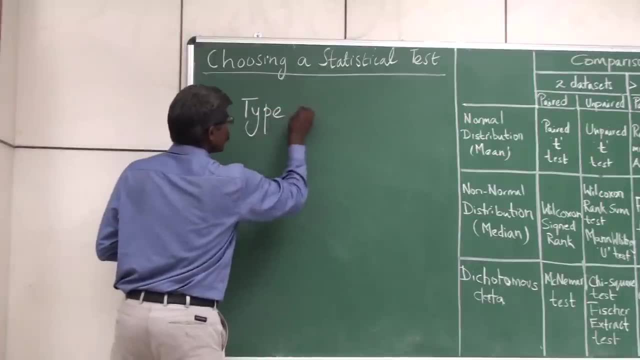 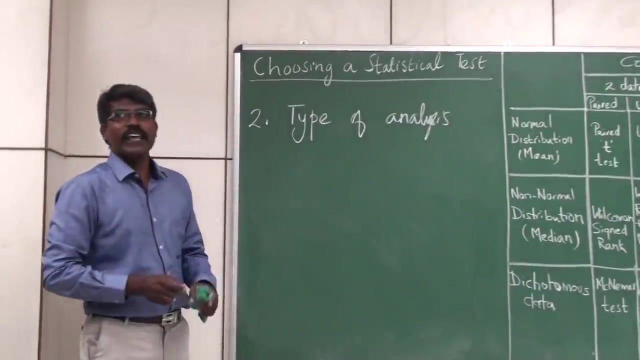 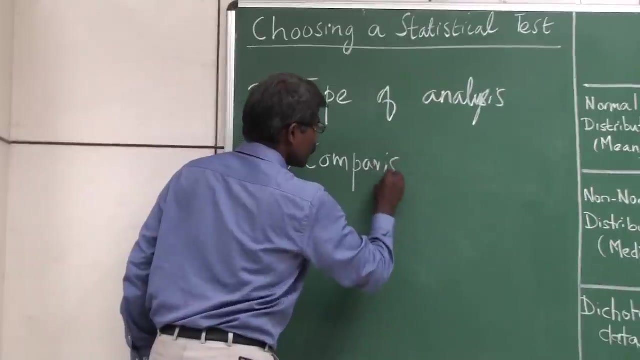 factor. The second factor which we need to know is: what is the type of analysis we want to do? Again, it can be of three types. The first, subduation, is we can compare two or more groups, So it's a comparison. The second subtype is: we can compare two or more groups, So 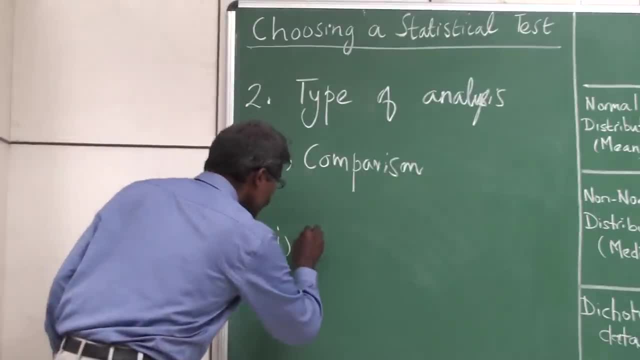 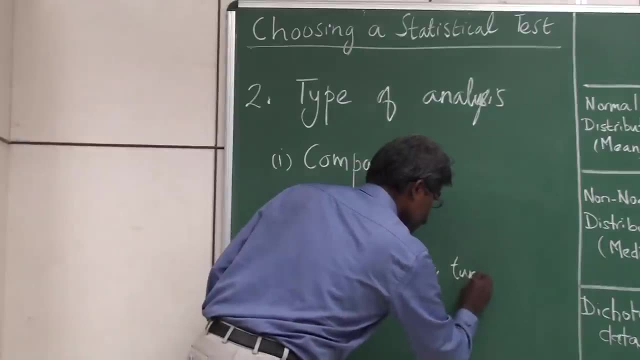 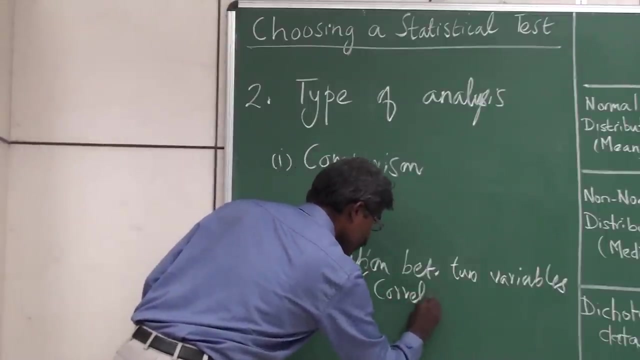 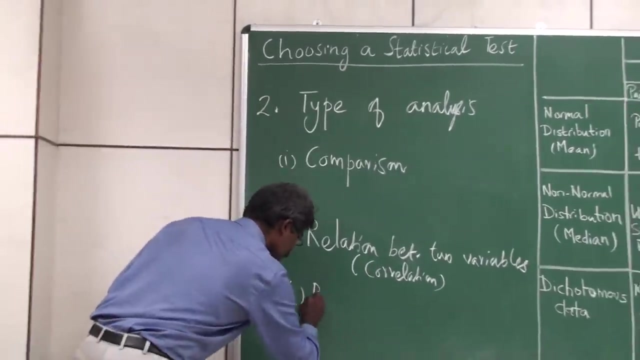 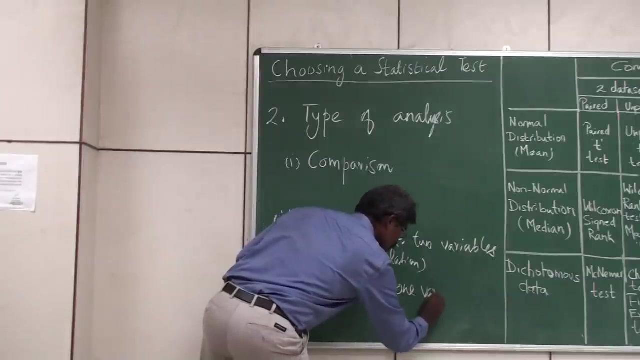 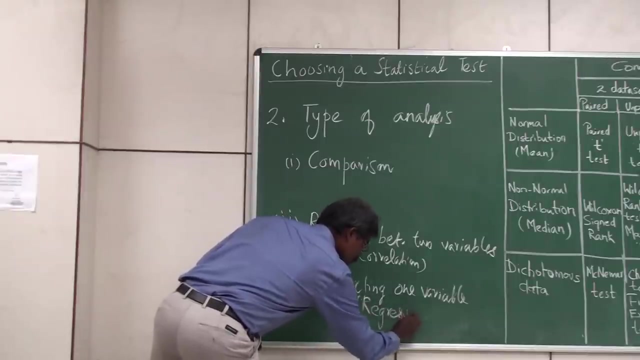 the third subtype is: we want to find out the relation between two variables, which is called as correlation. The third type of analysis can be predicting one variable from other. This is called as regression. Now let's take one one by one. Comparison can be comparison. 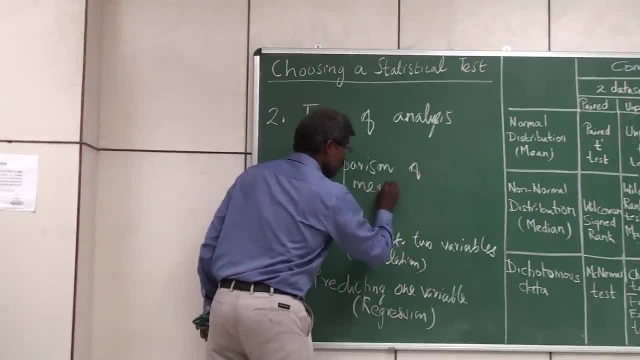 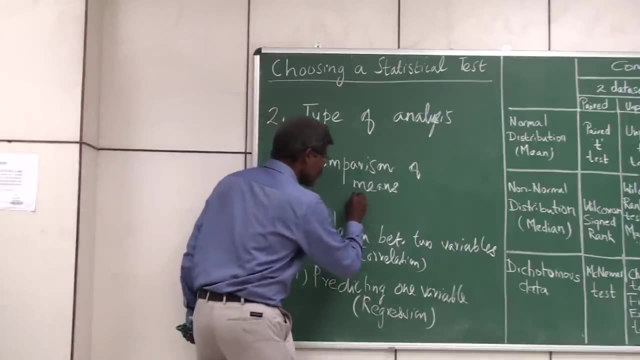 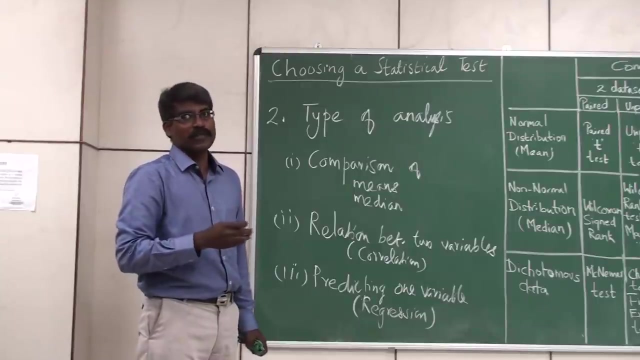 of means. If our type of variable were continuous, numerical, then we will be comparing means. It can be comparison of medians If it is a numerical, continuous variable, because this is the our type of analysis variable but does not follow normal distribution. the classical example i showed us: vasco or abacar. 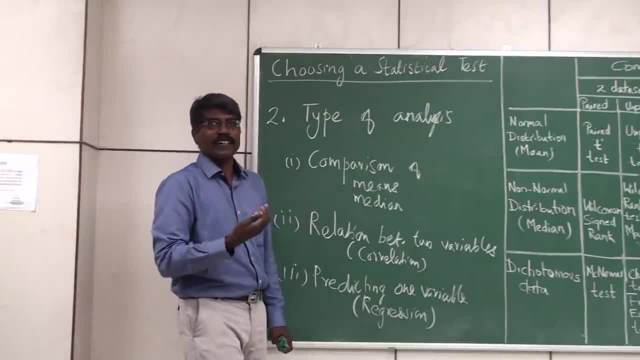 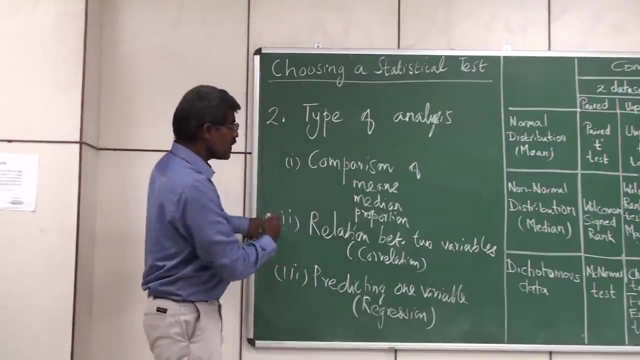 score or if it is a dichotomous data, it will be comparison of proportion between two groups. so comparison can be either comparison of me, comparison of median or upwards of proportion. so we need to fix any one of these. the second type is we have one group but two variables. we 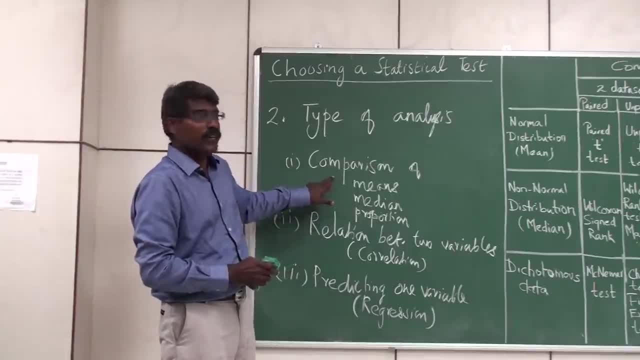 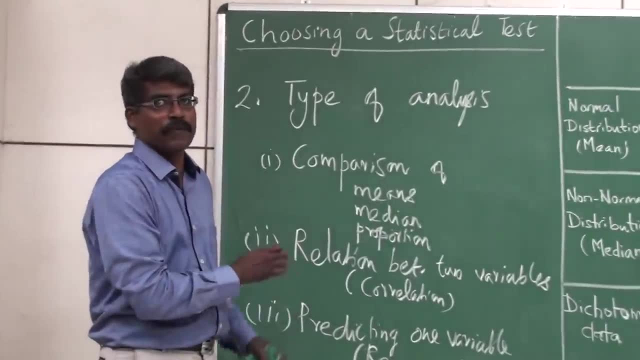 are measuring. we don't have here we have two or more than two groups. here we don't have two groups, we have only one group, but we have two variables. let let me give a simple example to explain this. we are measuring body weight in one group of patients, say 50 people. we have in that 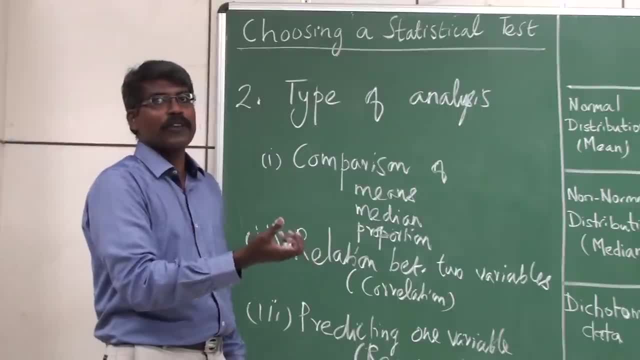 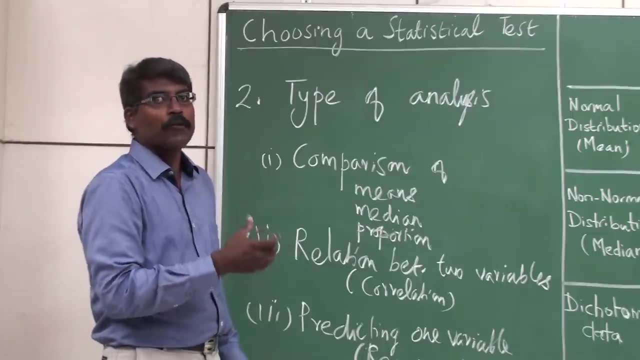 50 group of people, 50 people in one group. we are measuring body weight- the same group. i am also measuring blood pressure. now i want to know whether, as body weight increases, blood pressure increases. or as body weight increases, blood pressure decreases. so i want to find out. is there a relation between these two variables? so please remember these two variables. 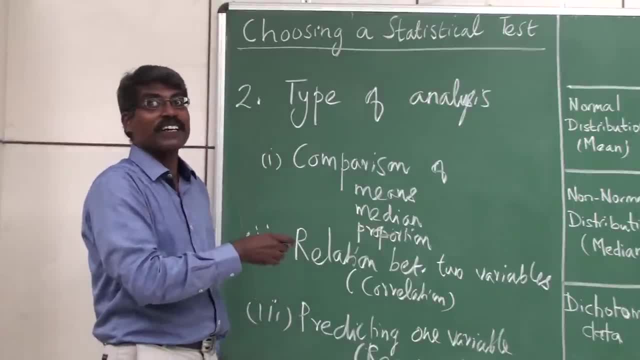 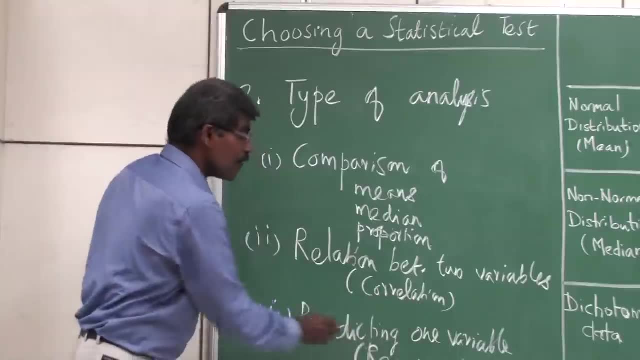 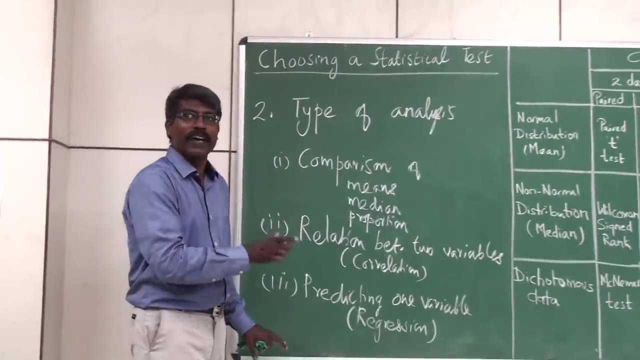 are measured in the same subject in that one group. so we have only one group here. now the third type of analysis is predicting one variable from the other, which is called as regression analysis. again, this is also very simple. here again, we have only one group, but we have only one group. 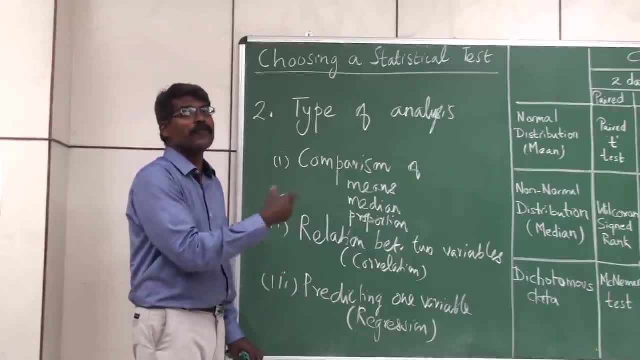 now here i want to predict one variable from another. say, for example, if a person of 50 kilo comes to my outpatient department, what would be his blood pressure, if i want to find out that mathematically it becomes predicting one variable from other. so i want to predict blood pressure. 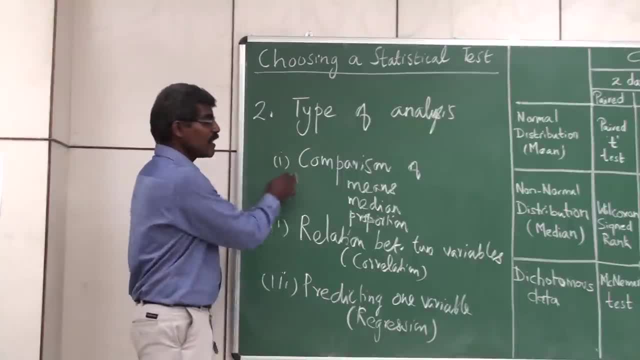 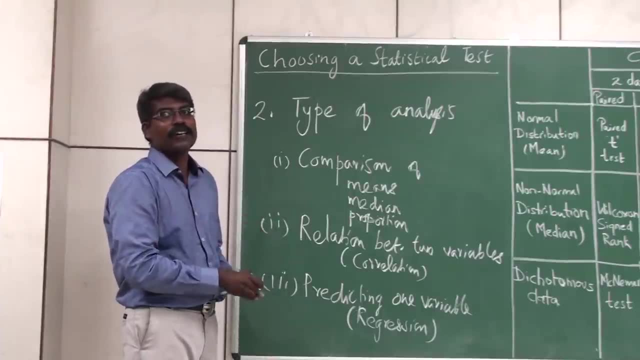 from the body weight which i have measured in this. so these are the three different types of analysis, so we need to fix any one among that. so that will be the second step for doing the statistical test. right now let's look into the third type, third factor. 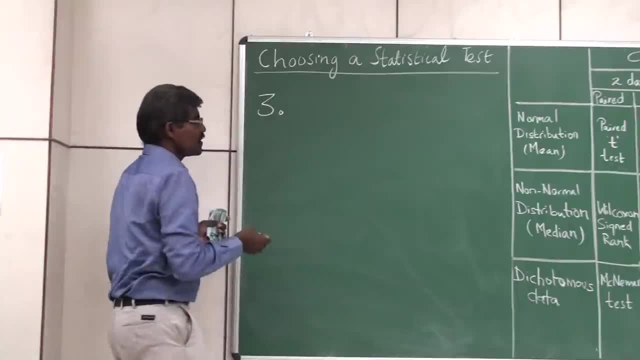 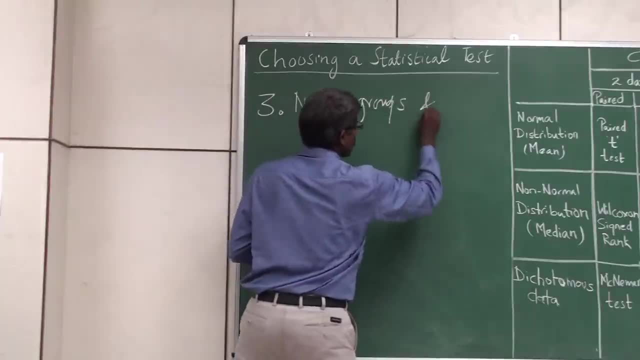 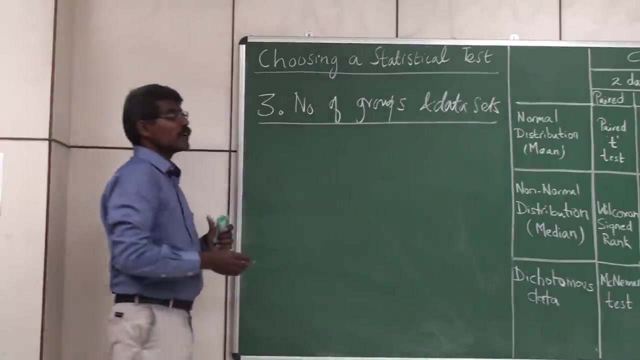 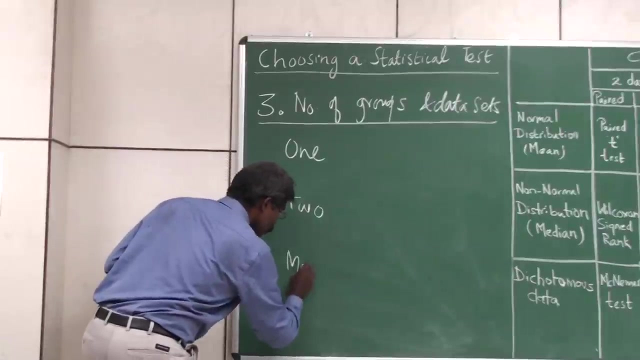 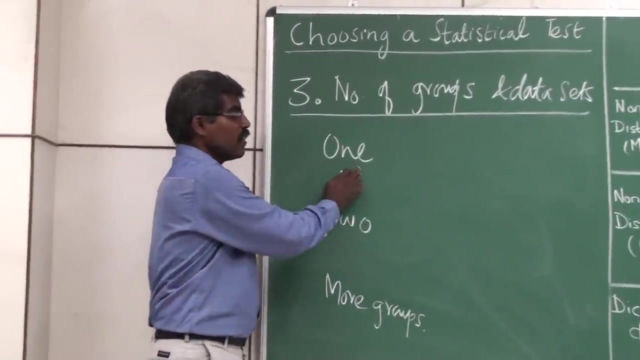 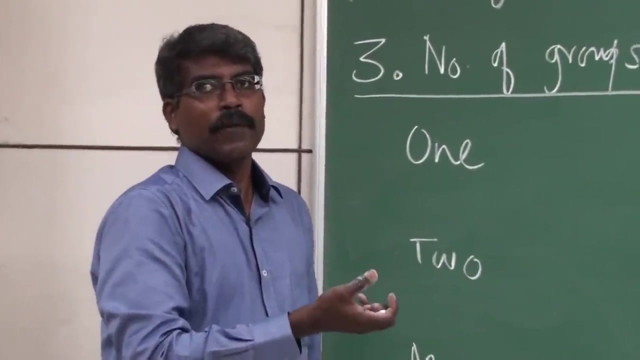 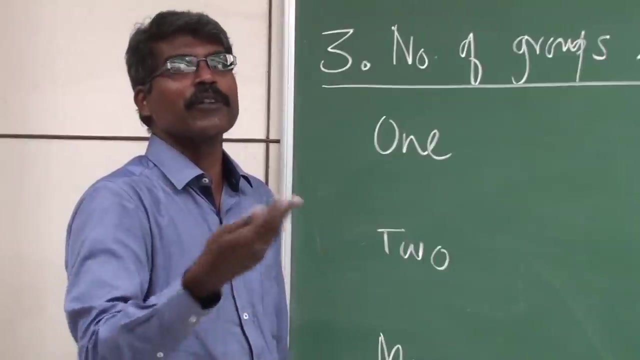 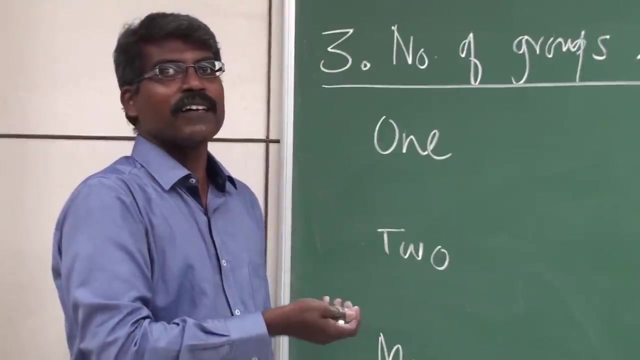 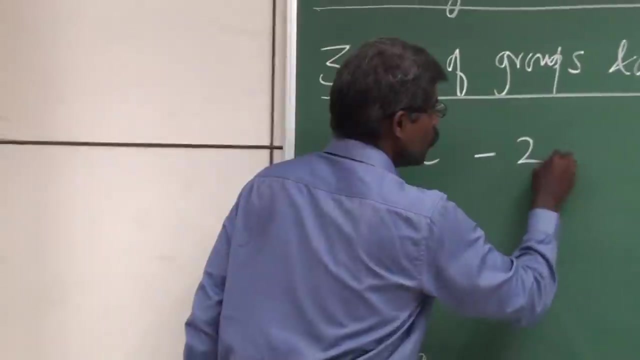 the third factor which dictates the selection of statistical test is the number of groups and data cells. I have only one group. all the measurements I am doing, I have one baseline data, intervention, then post-intervention data. So here one group, but I have two data sets. 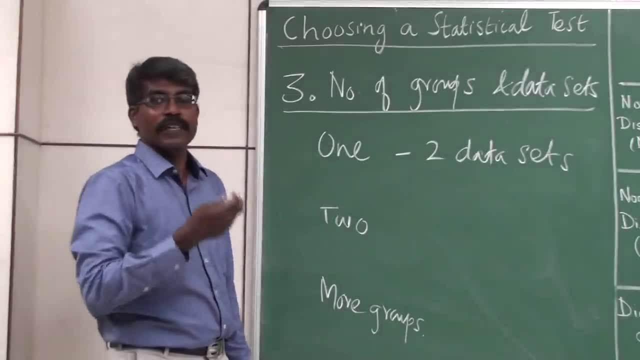 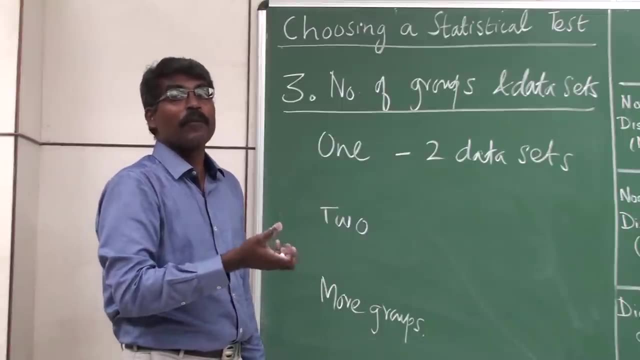 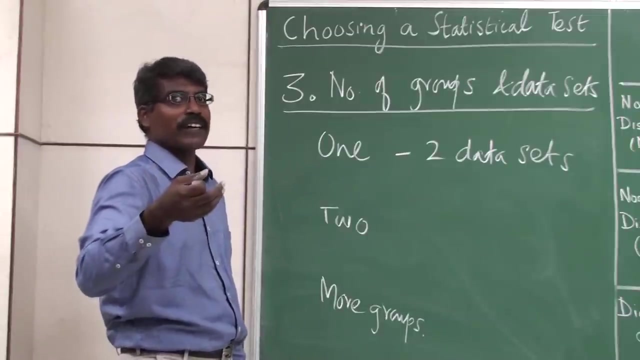 This can be one type, The same thing. I have only one group, say again 50 hypertensive patients. I give an anti-hypertensive but I measure blood pressure after one hour after the drug, six hours after the drug, 12 hours after the drug and 24 hours after the drug. 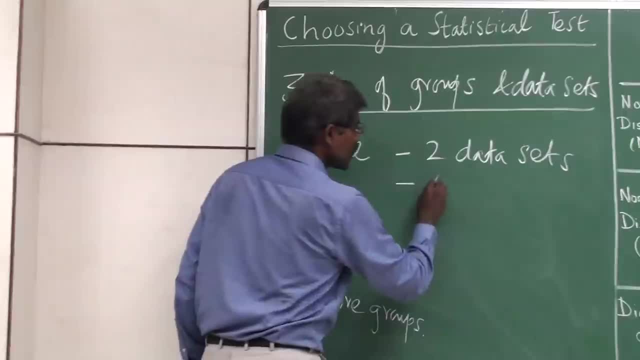 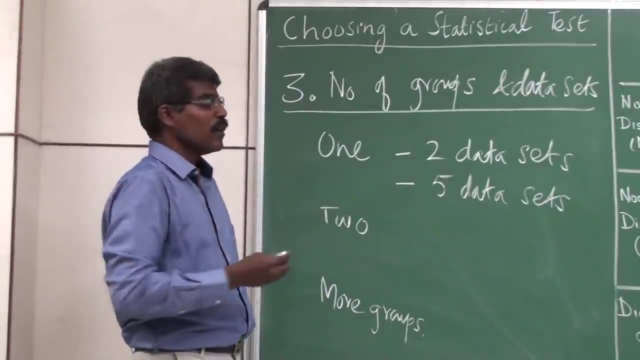 So now I have again one group, but at least five data sets, One at baseline and at four other time points. So this can be one, So one group, either two data sets, or one group more than two data sets. 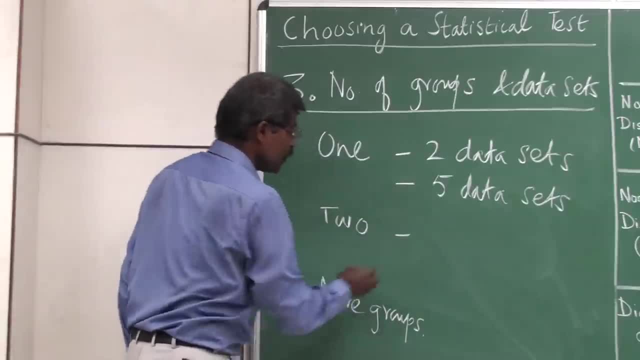 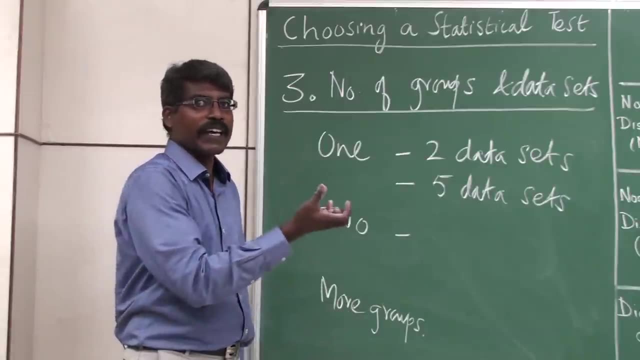 You need to fix that. The other way it can be two different groups. Let's take the same example of: I want to evaluate an anti-hypertensive. I take a group of 50 hypertensive patients. I give this new drug. 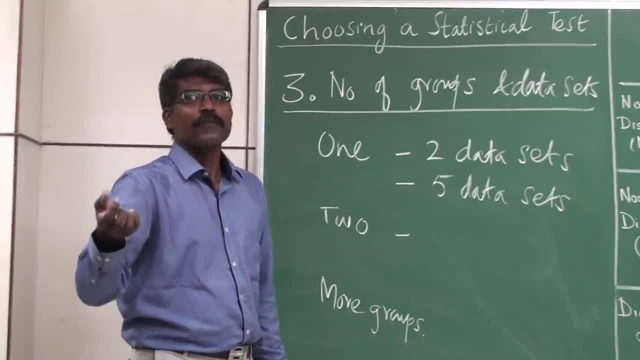 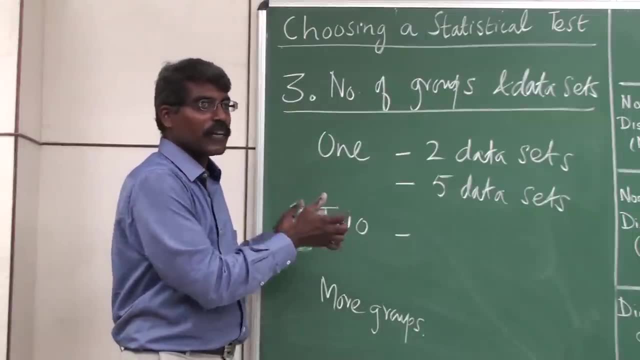 I have a totally different 50 set of 50 people hypertensives. I give a standard drug to them. Now you can see here this 50 is a totally different group which is not related to the first one. I have another group. 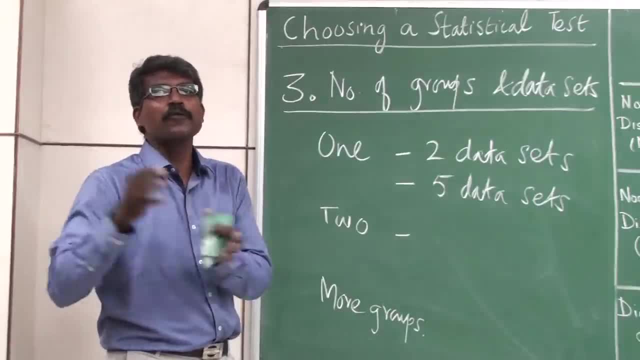 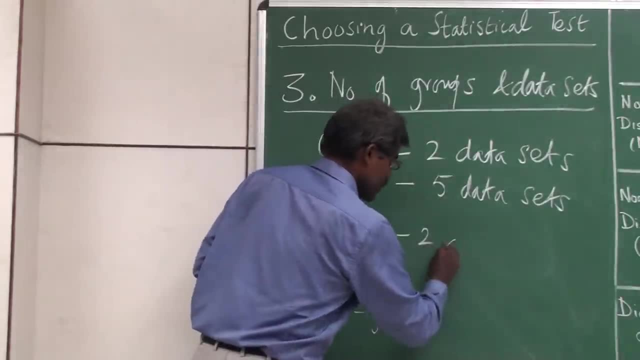 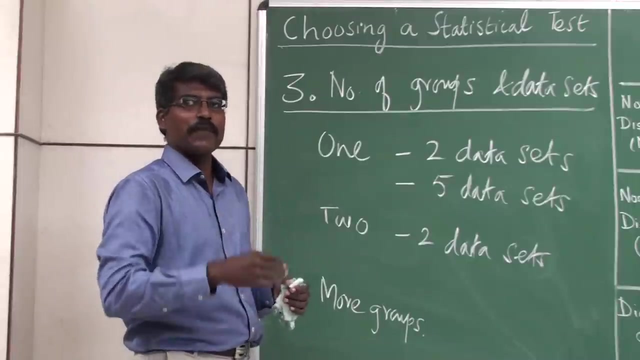 This is a group of 50 hypertensive patients. So these are totally two different groups and I get data from each. So I have two groups and two data sets. Now sometimes- let's take the same example- I have three group of hypertensive patients. 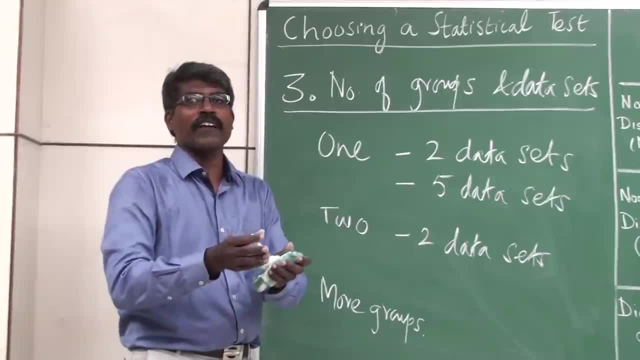 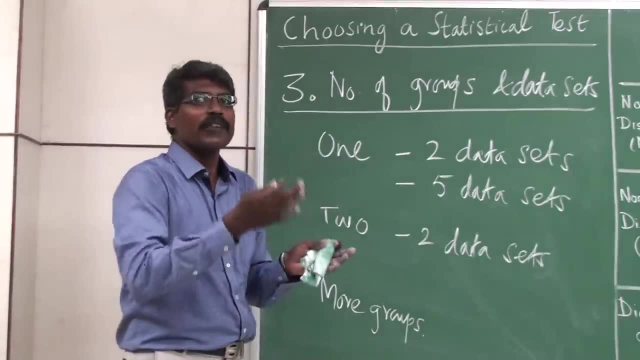 To one group, I give a new drug. To the other group, I give a calcium channel blocker. To the third group, I give an anti-hypertensive. To the fourth group, it might be diuretics. So I have more than two groups. 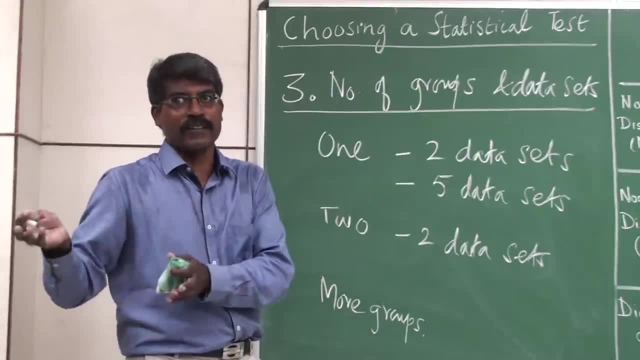 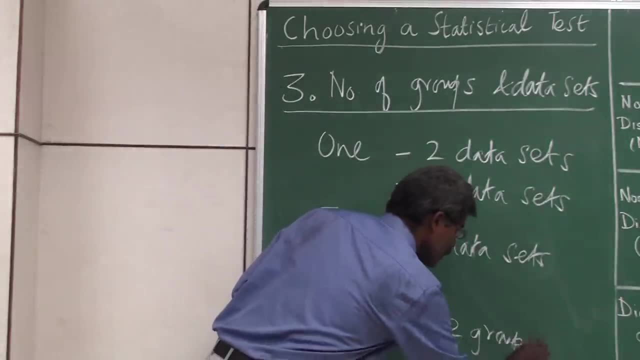 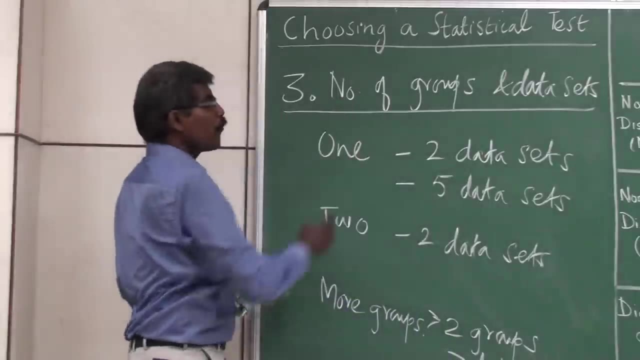 Here, in this case four groups, and all these four are totally different. So this is an example of more than two groups and I have more than two data sets. So the third factor is number of groups, and you need to fix any one of these. 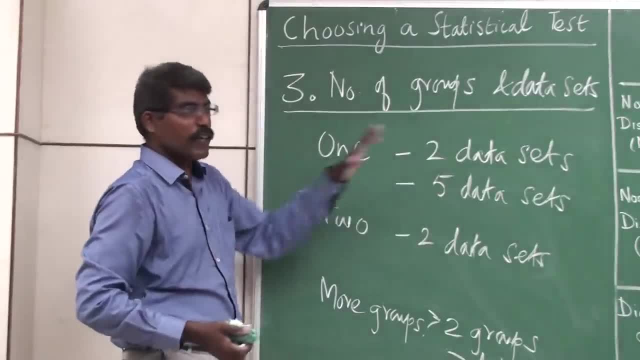 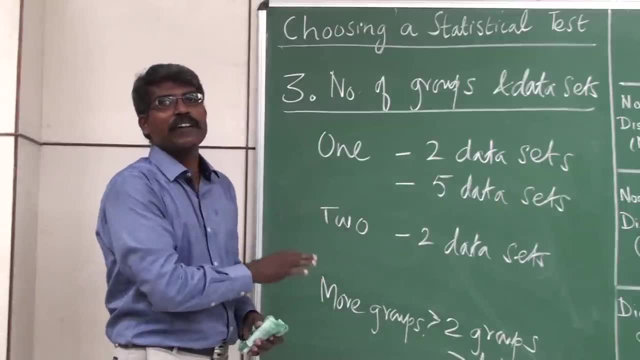 Do I have one group and two data sets, One group and more than two data sets, Two groups and two data sets Or more than two groups and more than two data sets? So that's the third factor which you need to fix in to select which statistical test you want to do for analysis of data. 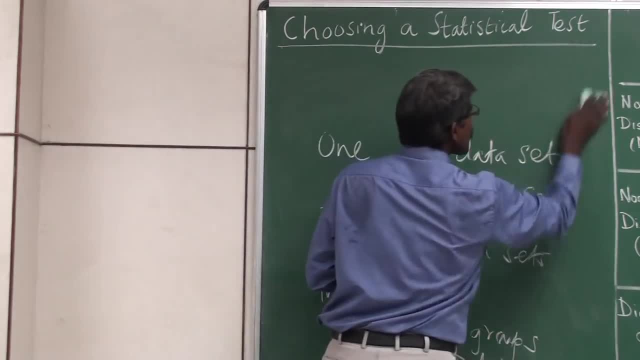 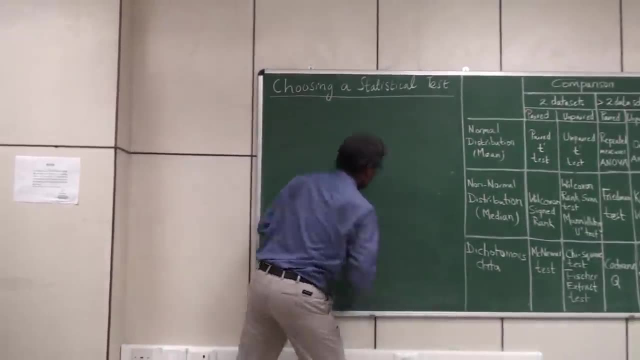 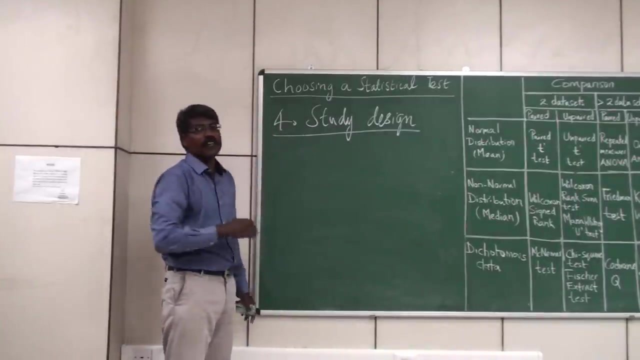 Now let's go into the fourth factor, which dictates the selection of statistical test. The fourth factor is the study design. Now, in scientific research, all of you have read about study design. There is a lot of various study design: Craft, sectional case control, COVA, RCT. 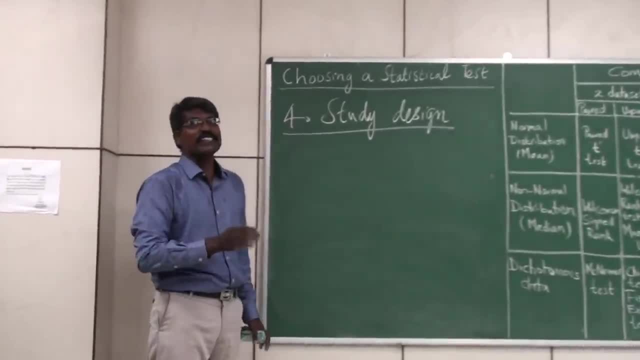 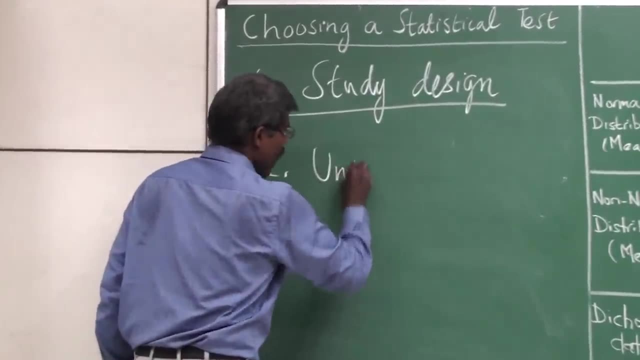 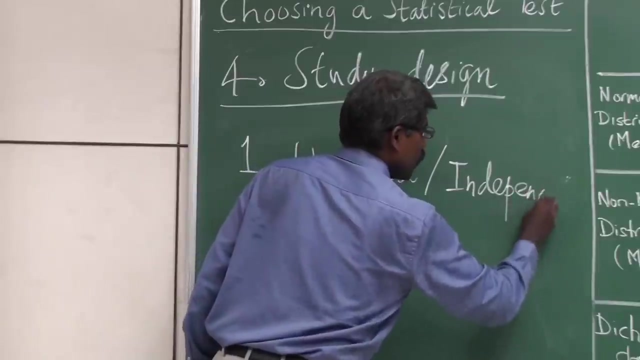 In terms of statistics study design. we mean there is only two types of study design. Please remember that The first one is called as unpaired, Or some people call it as independent. What does this mean? Again, please remember this word independent. 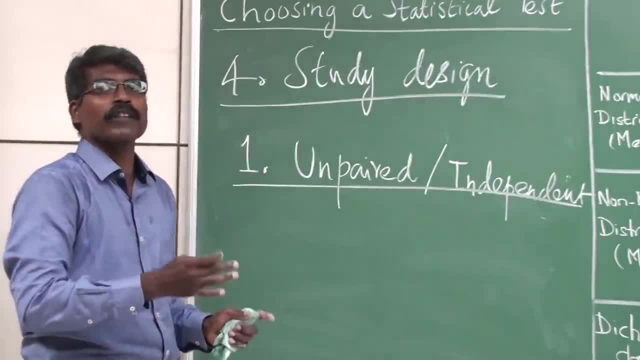 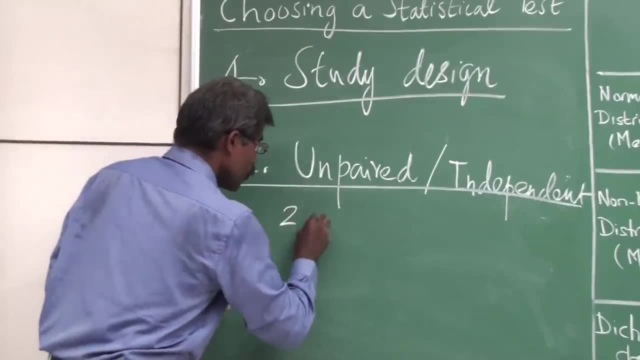 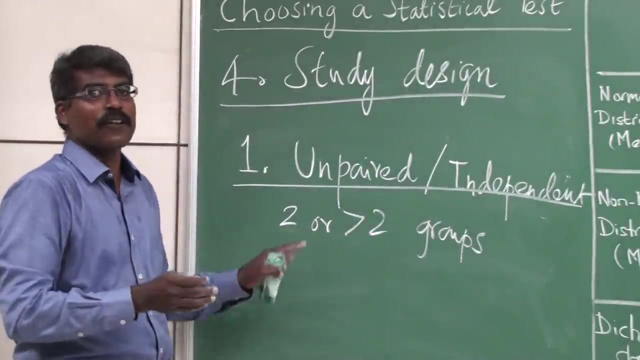 It's very self-explanatory. There are two or more than two groups which are not related to each other, Which are independent. So here we have two or more than two groups of totally different set of subjects. So that's called as unpaired design. 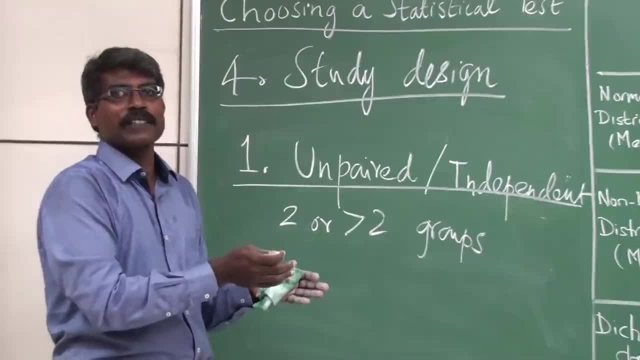 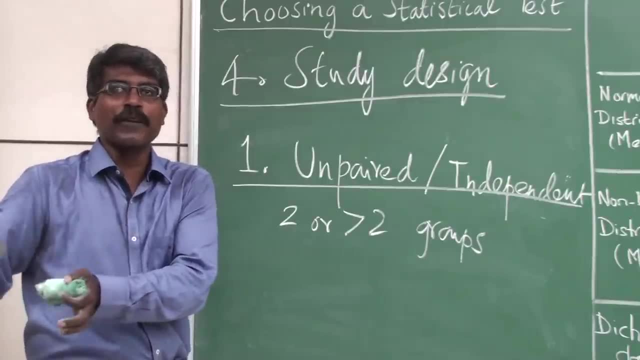 To quote an example, If I give one group of 50 hypertensive patients, I give one rep. To the other 50 hypertensive patients belonging to a totally different 50 people, I give another. So this is a classical example of unpaired design. 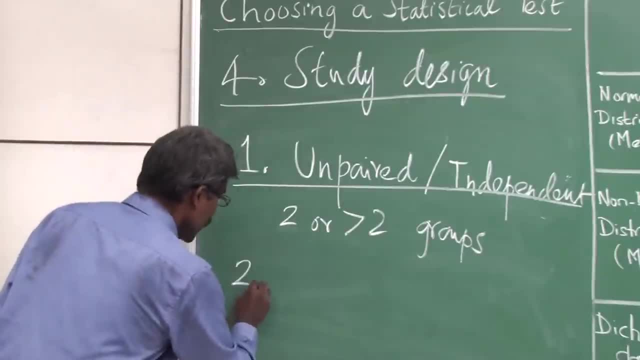 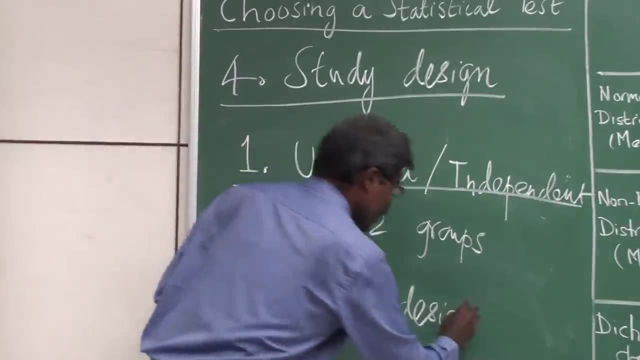 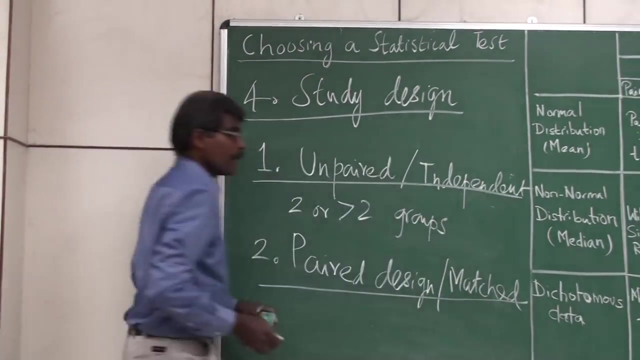 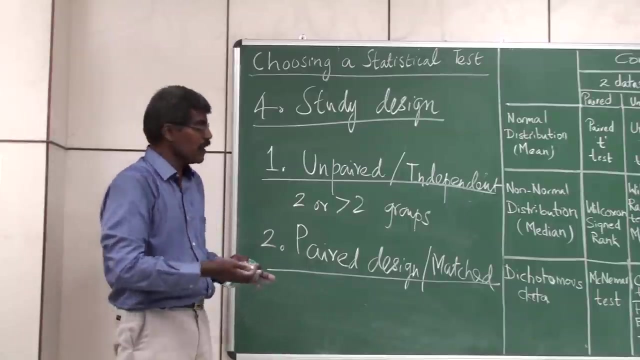 Or independent design Or unmatched. The second type of design is called as paired design Or sometimes called as matched. Again, This is very self-explanatory. The readings which are got from this group are matched to each other. So what do we mean? 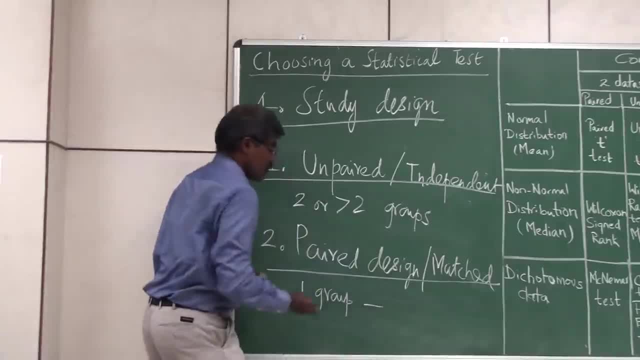 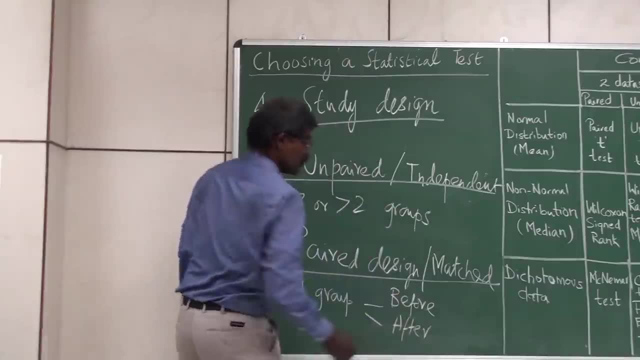 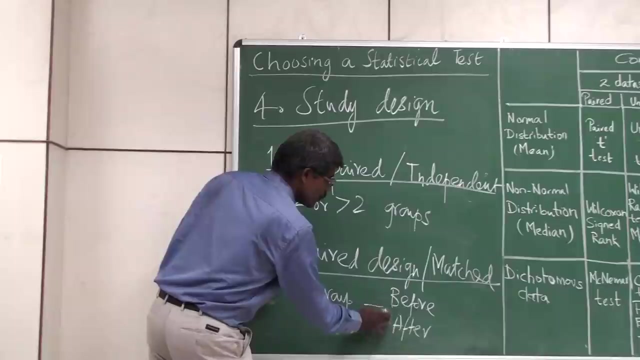 I have only one group. Before giving a drug, I measure, And after giving a drug, I measure. So I have two data sets: One group, two data sets. So this type of design is called as paired design: These two data. 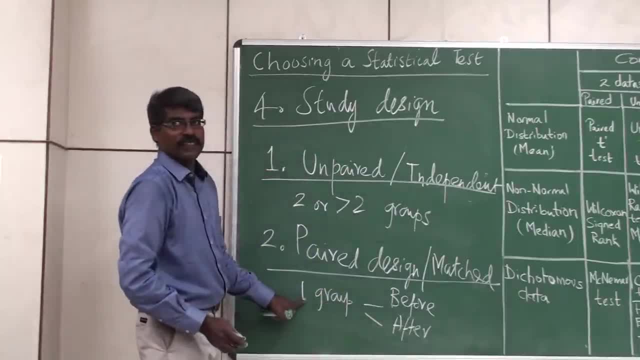 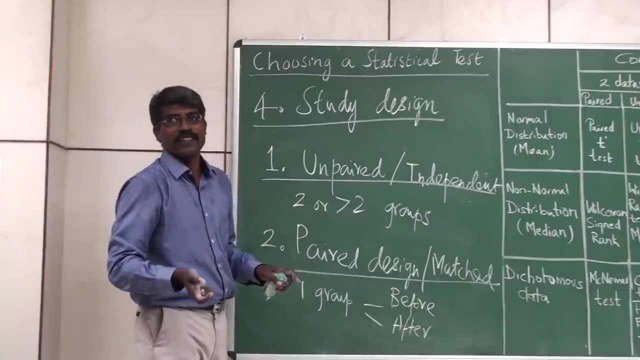 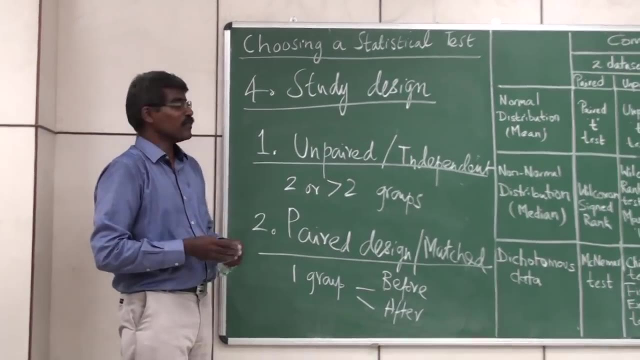 are paired to one single subject. They always go as a pair. You cannot put before data of one person to after data of someone else, Right? So that's why this is called as paired, Or they are matched to each other. That's why it's called as matched design. 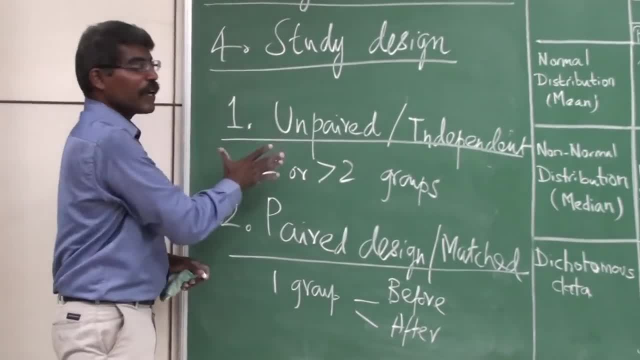 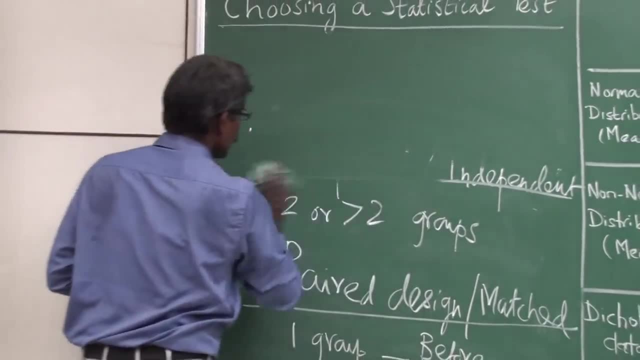 So that's the fourth factor which you need to decide: Is it a paired type of design Or is it an unpaired type of design? The last type, The last factor which we need to consider before we go on into the selection of statistical test, is: 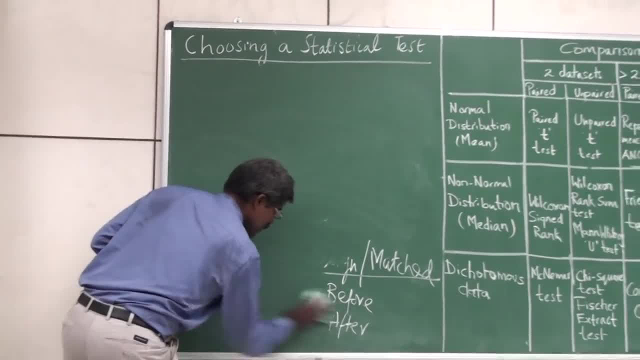 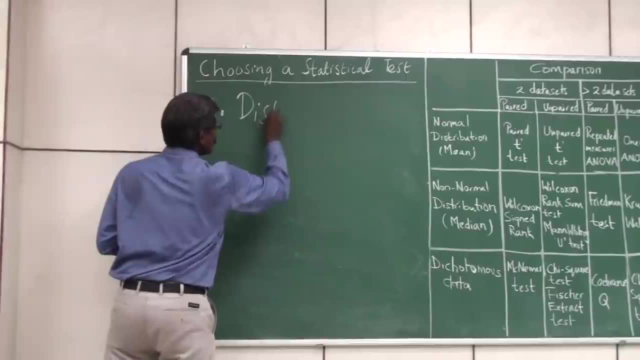 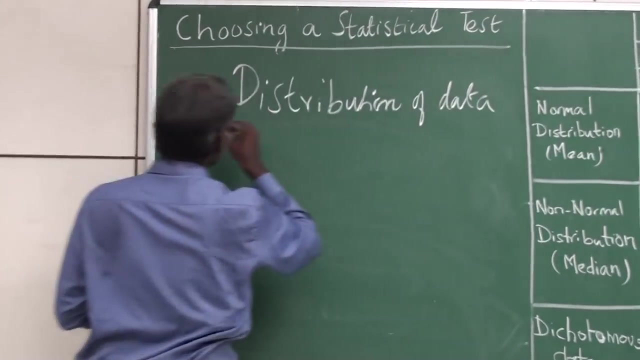 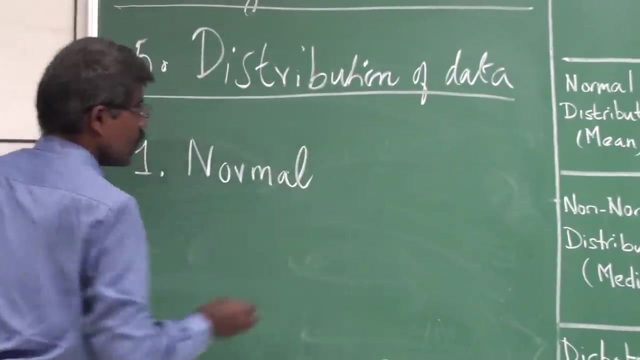 before we go on into the selection of statistical test. is So the fifth factor? So what is the distribution which we need to find out? is distribution. Again, we need to fix whether it follows normal distribution. Again, we have seen the rule of thumb. 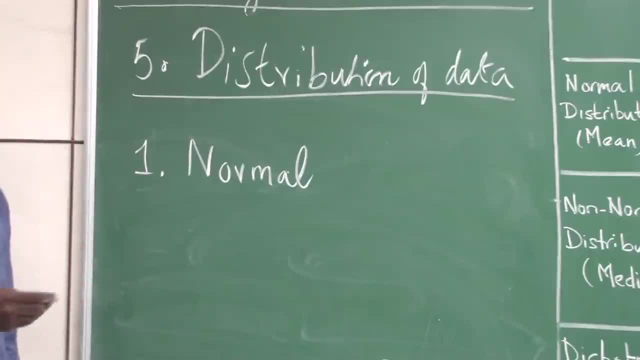 All body parameters follow normal distribution, except a very few like antibody titer. So bodily parameters like blood weight, blood pressure, glucose, cholesterol level, all these things are classical examples. Or does it follow non-normal distribution? Classical examples of non-normal distribution we have already seen. 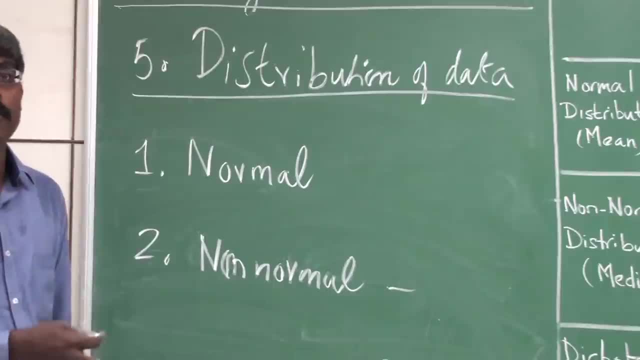 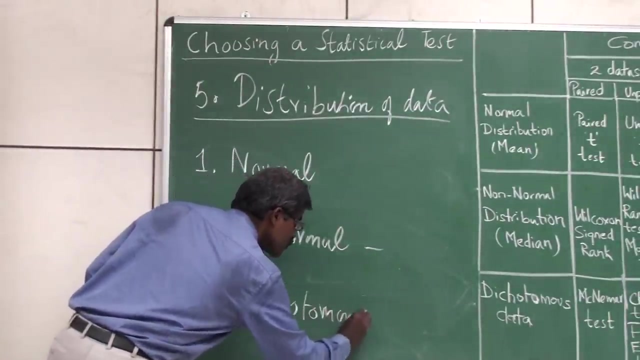 Any parameter measured as ranks or scores always or usually does not follow normal distribution. The third type: or is it a binomial distribution or dichotomous? Or is your data dichotomous Or, if you want, in terms of distribution it becomes a binomial. 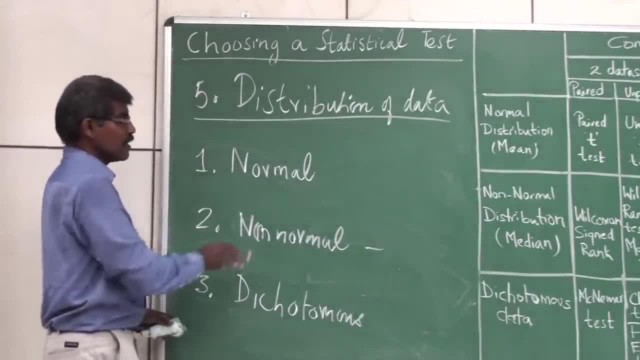 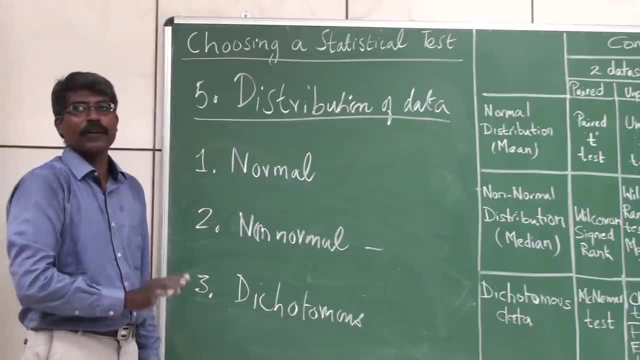 So you need to fix any one of these. Is it a normal distribution Or a non-normal distribution, Or is it a dichotomous type of data, binomial distribution? so any one of these three you need to fix now, if you. 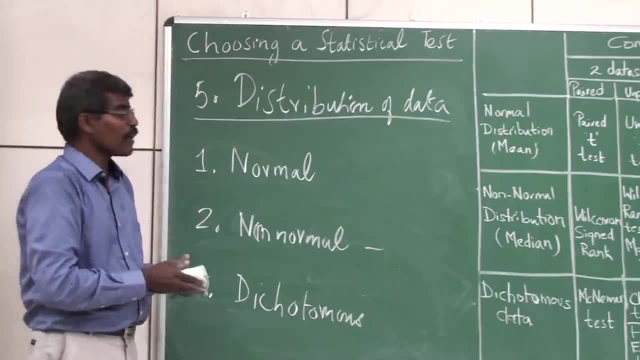 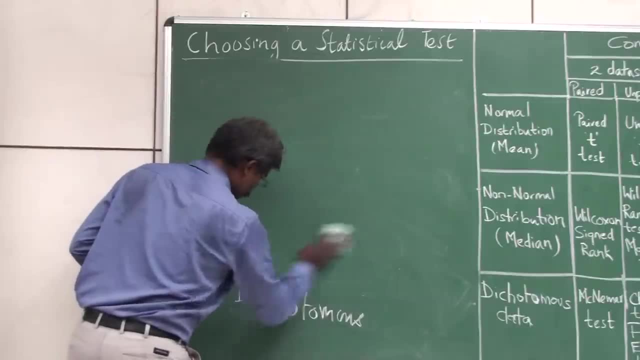 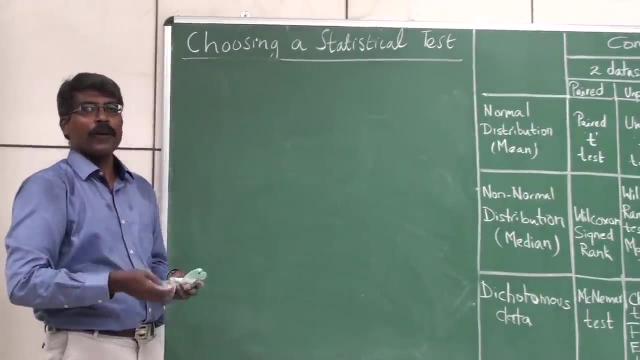 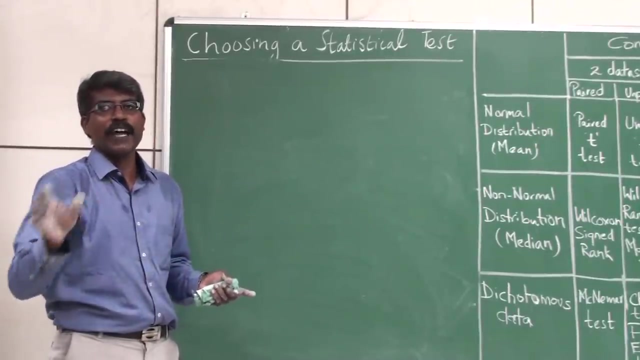 have fixed all these five parameters, it becomes very easy for you to find out which statistical test you need to select for analysis of data. now let's take a small example and try to work out this. let's take an example of: I have two group of fifty diabetic patients each. each group has 50 diabetic patient. they 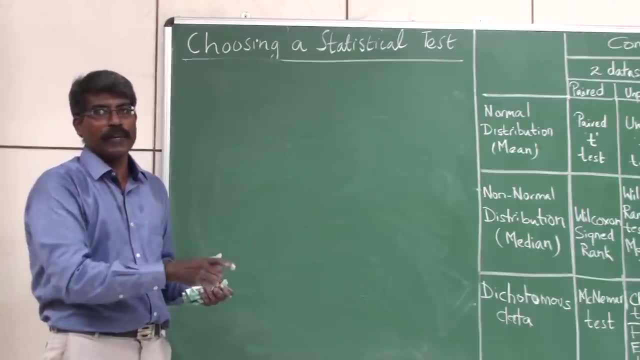 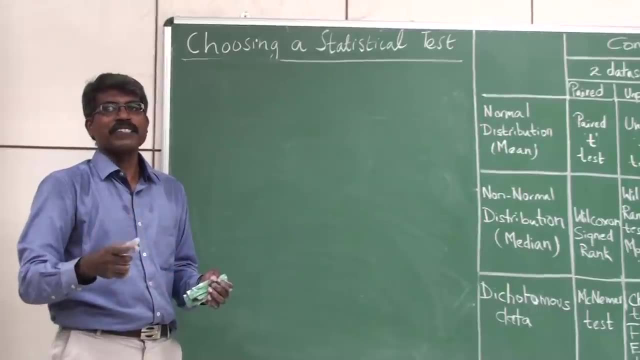 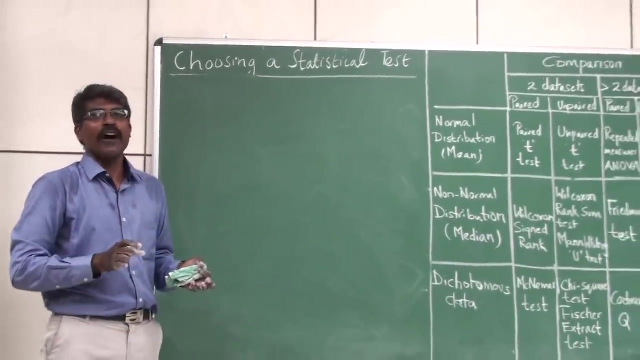 are totally two different groups. to one group I give metformin. the other group I am giving a new drug. I want to measure what is the change in the reduction in blood glucose level and find out: is the new drug more effective than metformin? let's take this is the scenario and I want to find out which statistical test 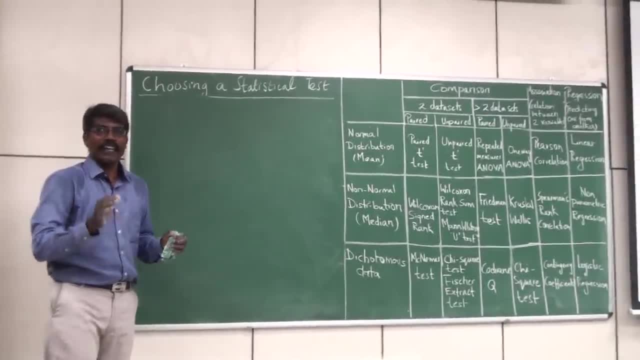 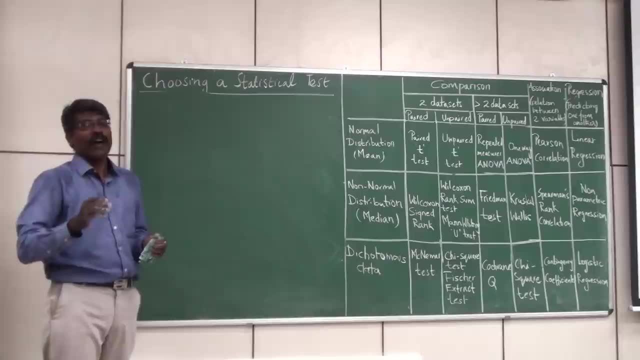 to be used for analysis of data. now again, there are several different input variables you could enjoy with. some of are five steps, which you need to go one by one, and if you fix this very, very easily, you can do. I will stress that please go stepwise, you will never be. 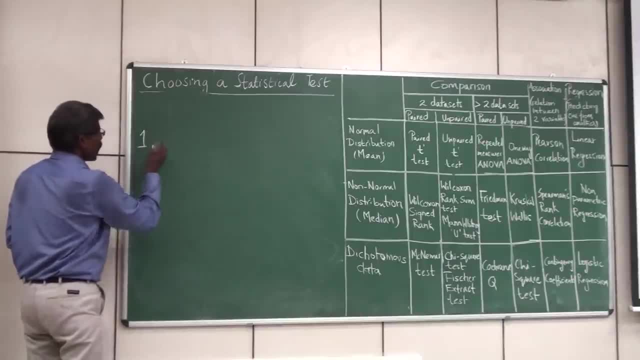 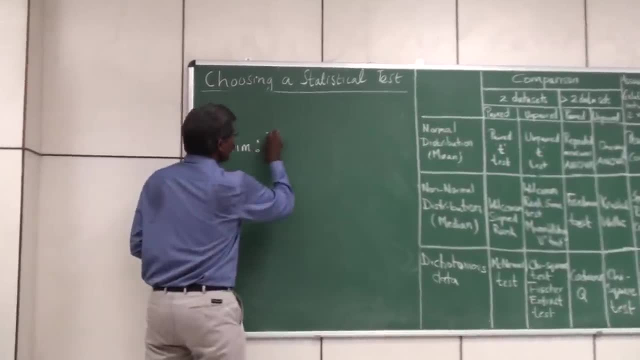 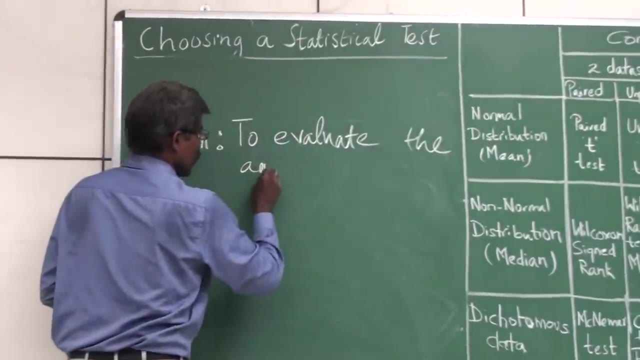 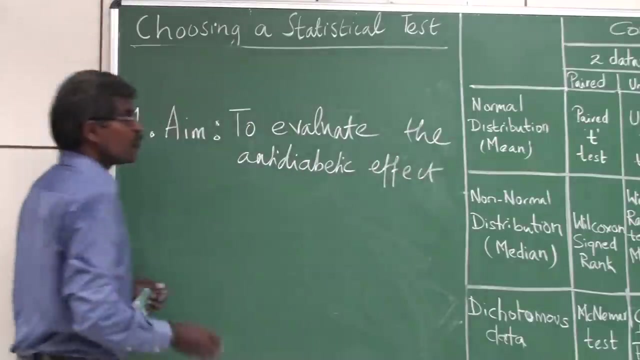 wrong. right, let's take each one, one, one, step by one. the first thing you need to write is: what is the aim of the study? now, here, the aim is to evaluate the anti-diabetic effect of youנים. so that's our a. the second step: what you 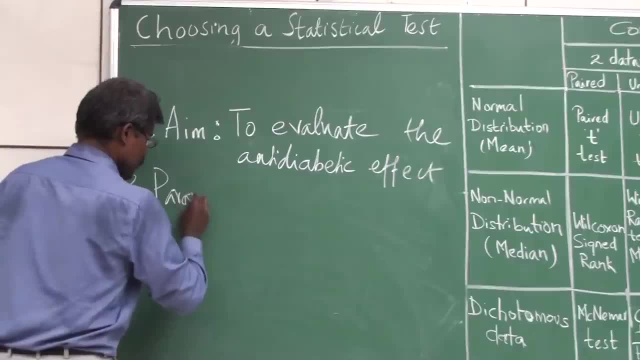 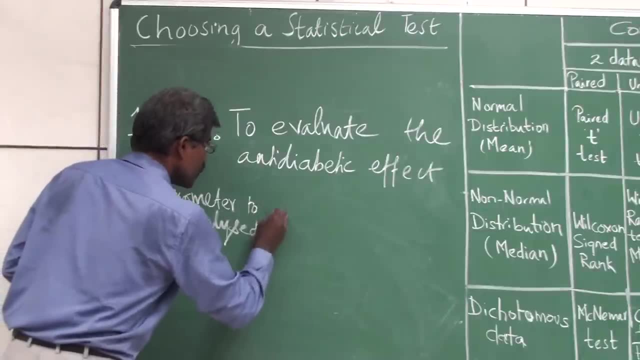 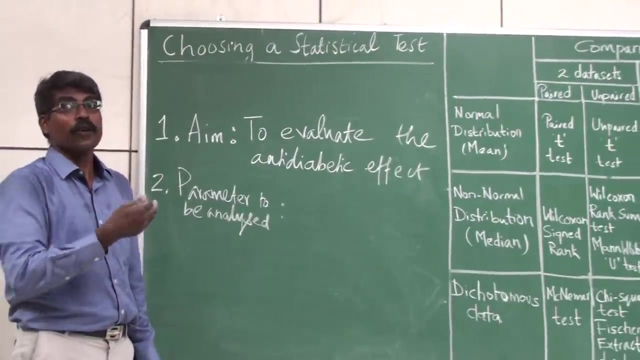 need to write is: what is the parameter you want to analyze? please remember that ugh file like this, we might have at least fiveを私個人ie is to be analyzed. so it goes without saying that for each parameter then you need to select which. 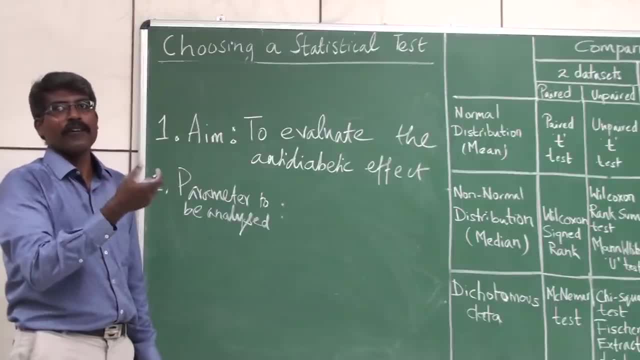 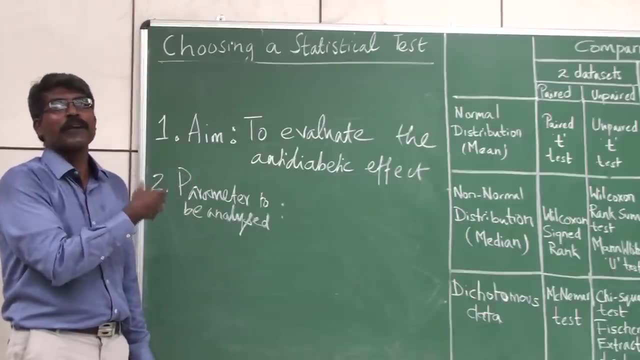 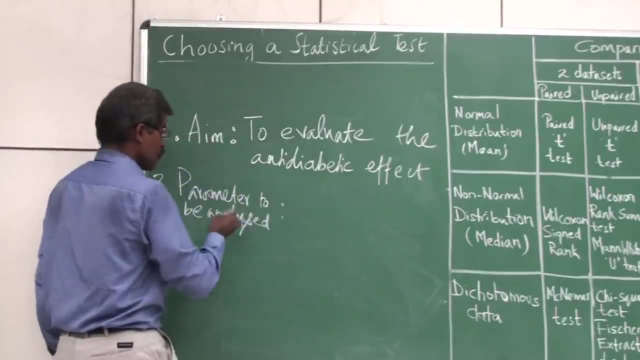 test to be used, as we told, like the ball, the weight of the ball, then we need some other tool. so if it is for the blood glucose level, it becomes thing. if it is number of people having adverse effect, it becomes anything. so here let's say I want to see the anti-diabetic effect. so what is the parameter? it? 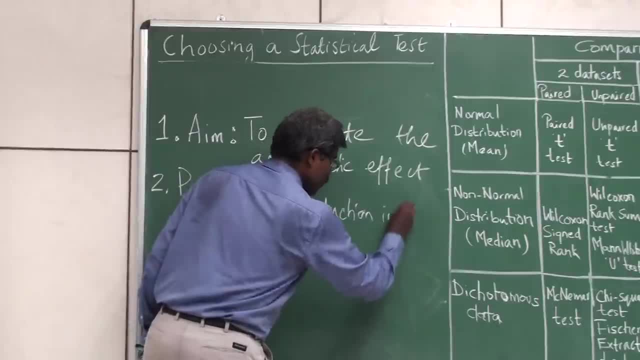 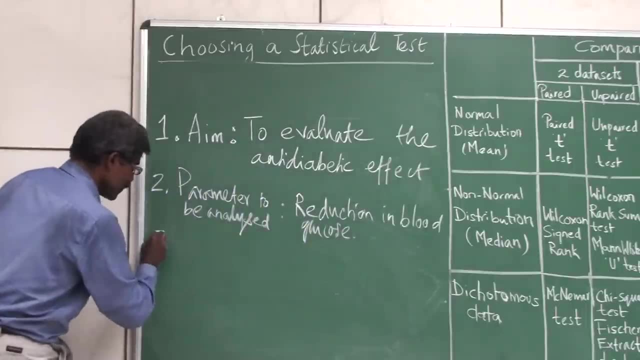 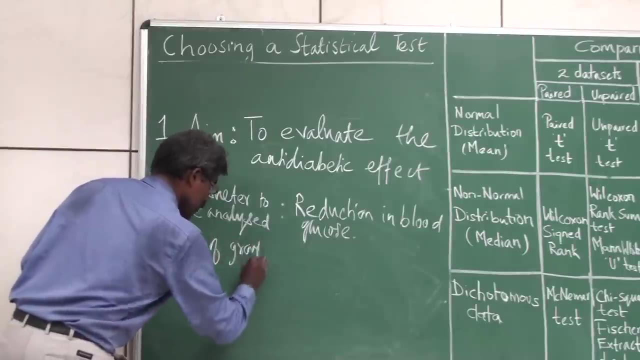 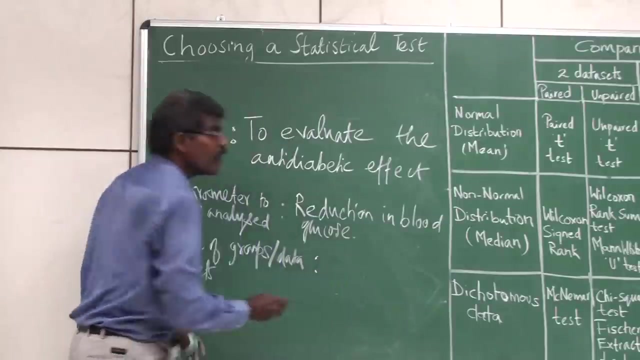 becomes the reduction in. the third parameter is number: number of views for data sets. and what are they now here? I told you we have totally two different groups, is it it so two groups and two data sets I have, is it it? you have two different groups, so two groups and two data sets I have, is it it? 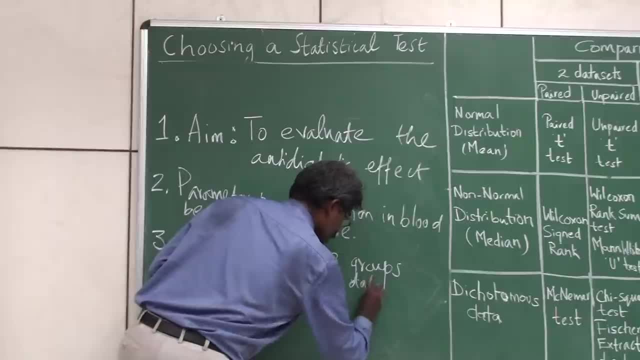 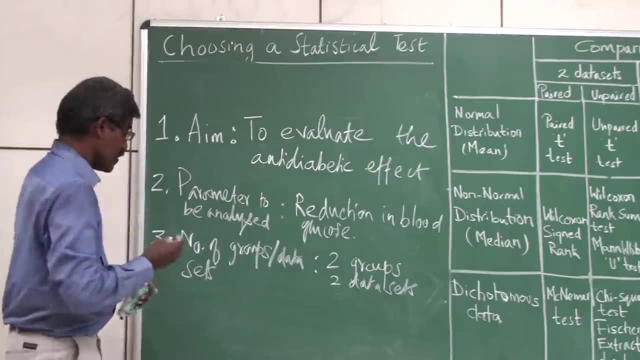 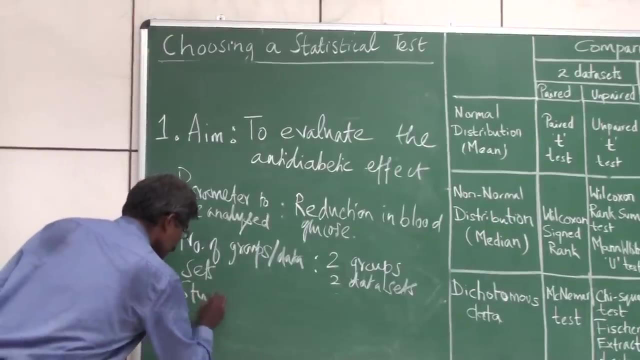 you have two different groups. so two groups and two data sets. I have, is it it? what are the groups? the first group is group receiving metformin. the second group is group receiving neutral. the fourth step which you need to do is: what is that study design? what is the study design in this example? they are totally 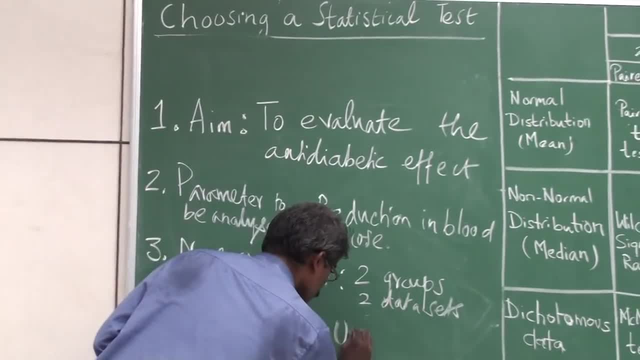 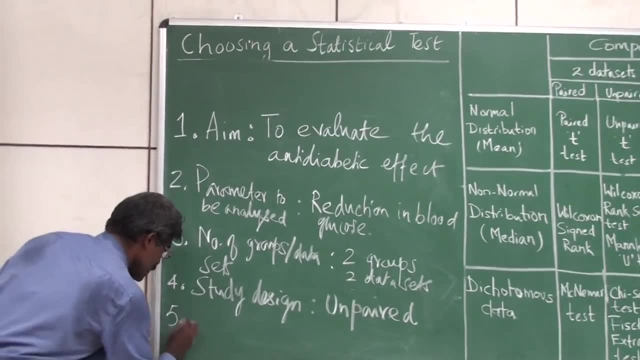 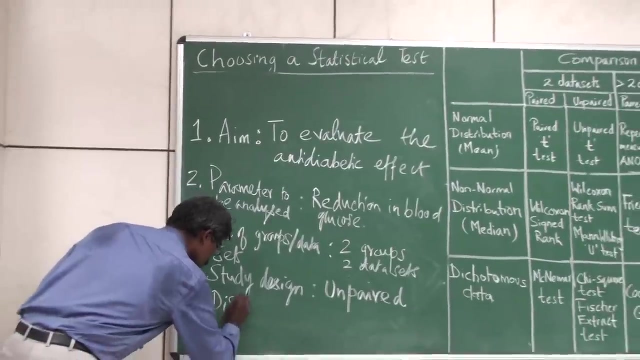 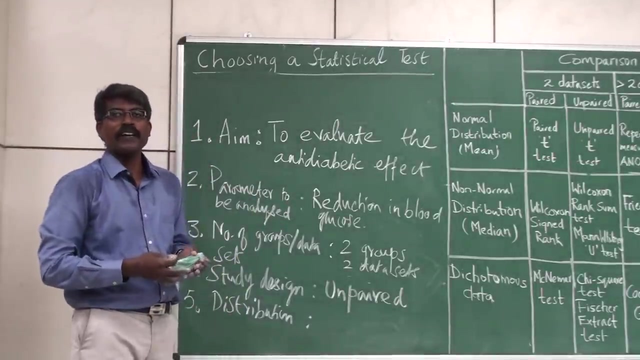 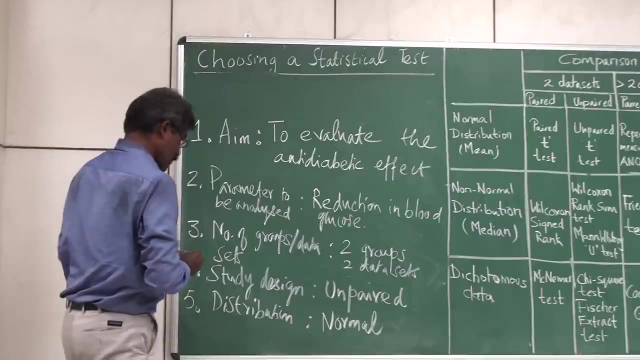 two different groups. so it is unfair. the fifth factor: as we have seen, we need to see what is the type of distribution, so the distribution. blood glucose is a body parameter. it follows normal distribution. there's a sixth factor which we need to write here: horse is what is the alpha pathways is? I'll just write it here: 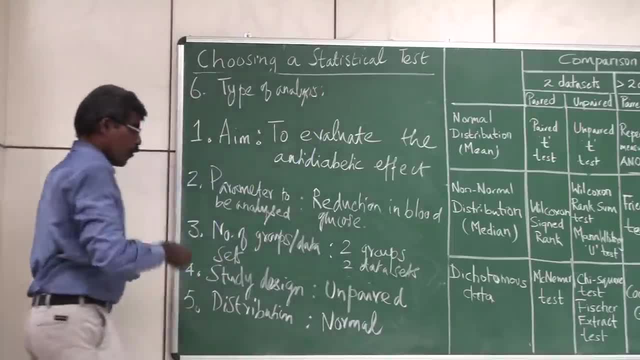 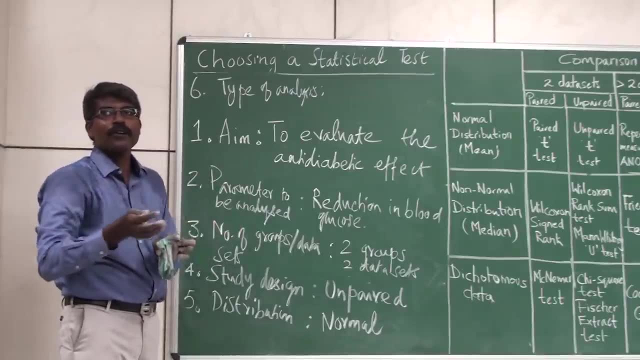 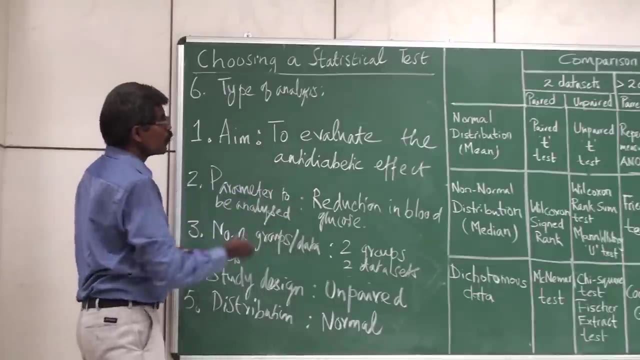 now here. we already saw that there are three major time sisters. fucker's a note or association, or regression, the strict correlation, or regression. now here we want to compare between two groups. so it is comparison, select. I don't want to predict or I don't want to find out. the 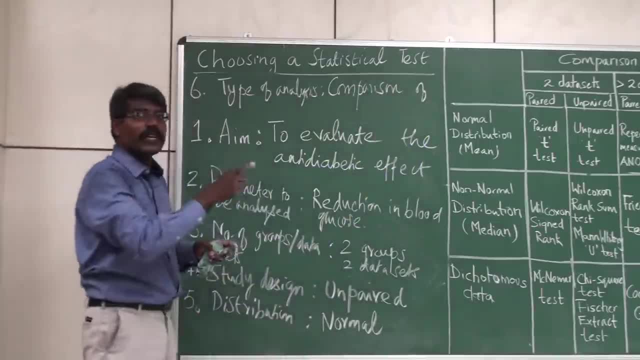 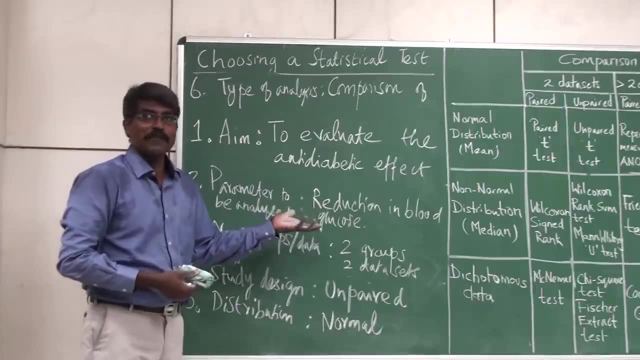 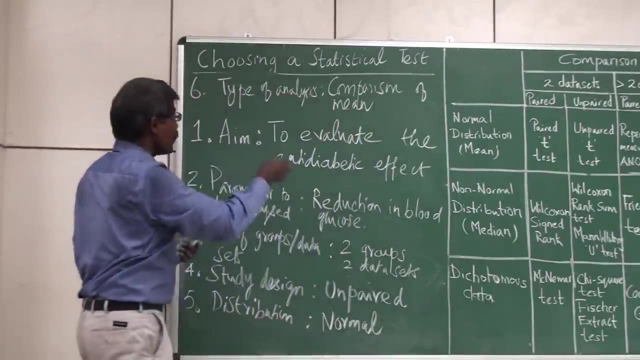 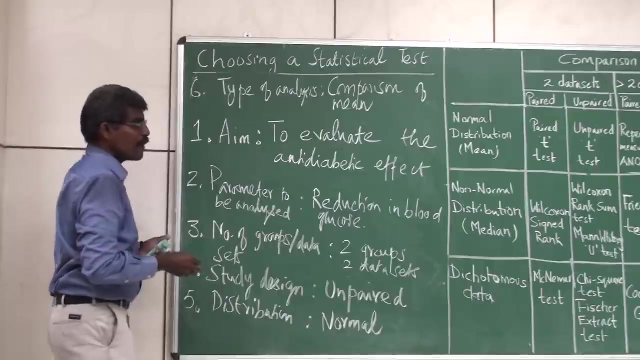 association. it's comparison of what. is it mean or median or proportion? what is my parameter? reduction in the glucose? how will I summarize it as means? so it is comparison of mean between two groups. so it becomes comparison of me, right? sometimes this is written third, doesn't matter wherever you write, it doesn't. 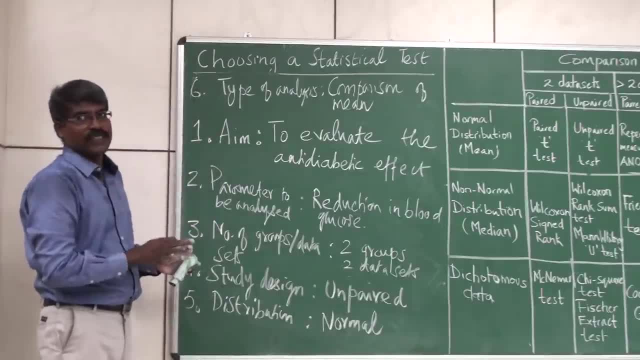 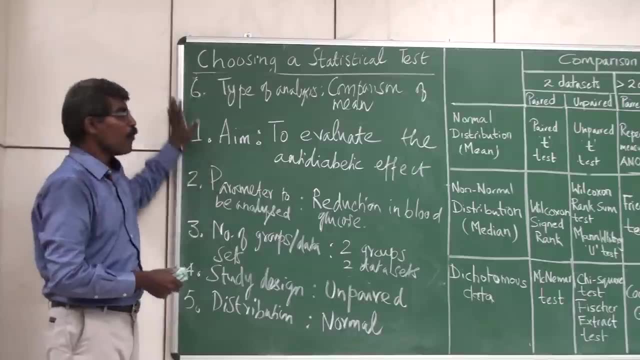 matter right. so these are the six steps which you need to fix or which you need to write. so I will urge you, please go step by step. you will never be wrong in that. now, once you have done that, let's look into this simple table which we 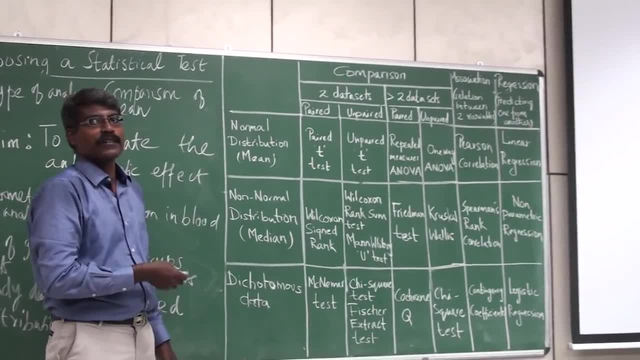 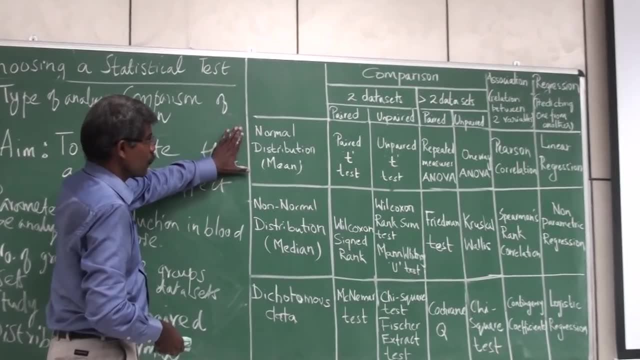 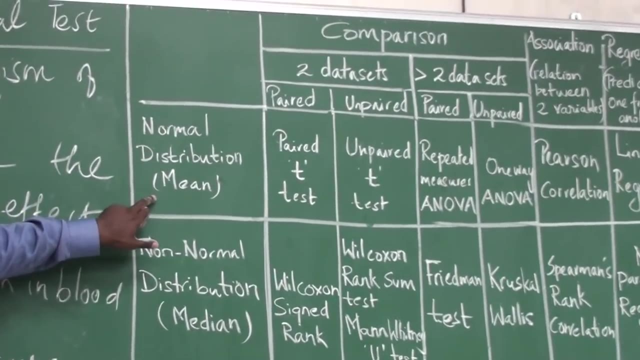 have reproduced from practical approach to postgraduate this PG dissertation, second edition of this book. now this table has three rows: row 1, row 2, row 3. let's first look into row 1: normal distribution, mean or comparison of means. second row is non normal. 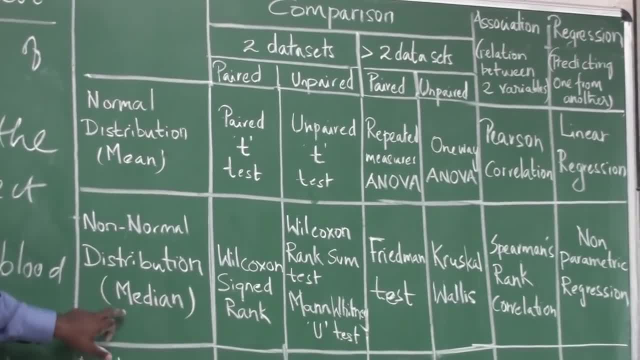 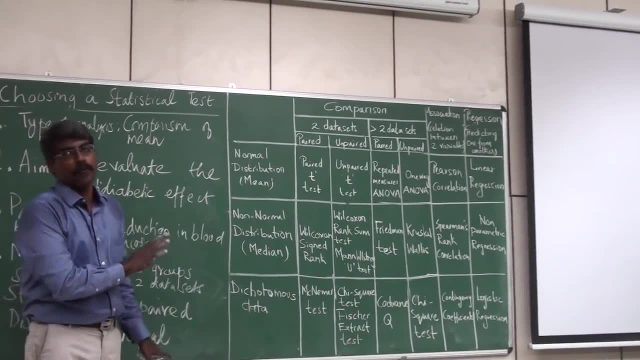 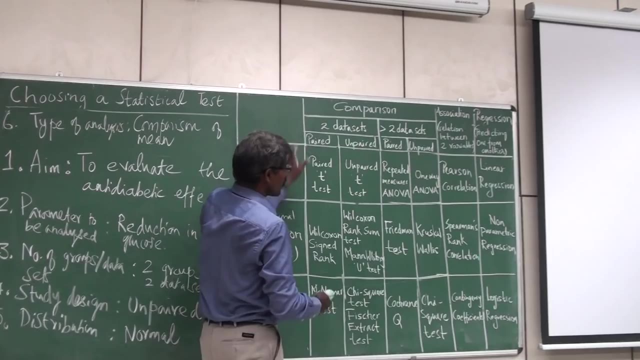 distribution where you want to compare, or variable, which are summarized as medians. third row is a dichotomous data which are summarized as proportions. now let's look into the column, now column. you can see you have again three major columns. this is one column and the next two columns. the first column, which is 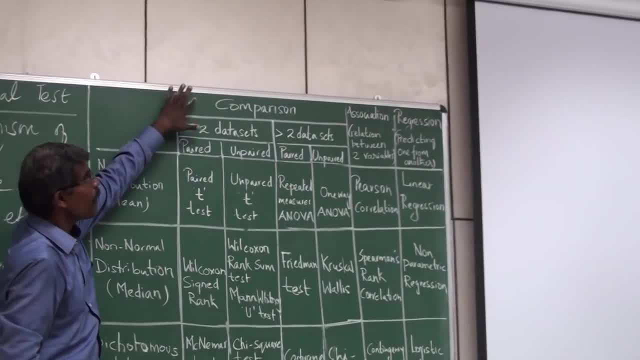 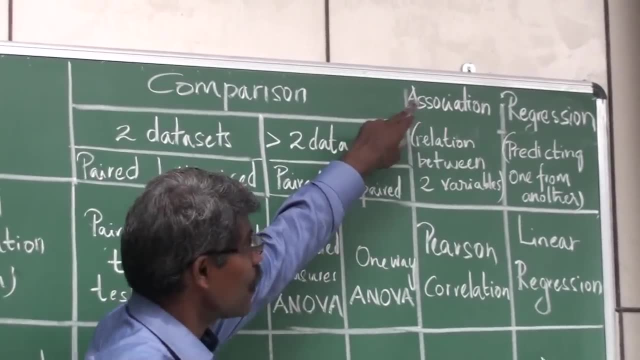 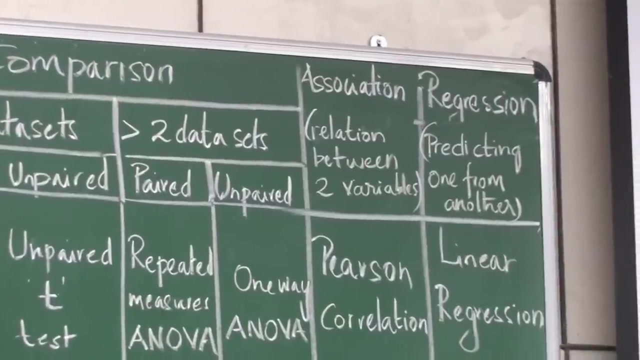 big, which has four subdivided columns, is comparison. so it is comparison of two or more data sets, isn't it? the second group, the second column, is association finding relation between two variables. the third column you can see is regression predicting one variable from one. now what we need to do is we need to fix the. 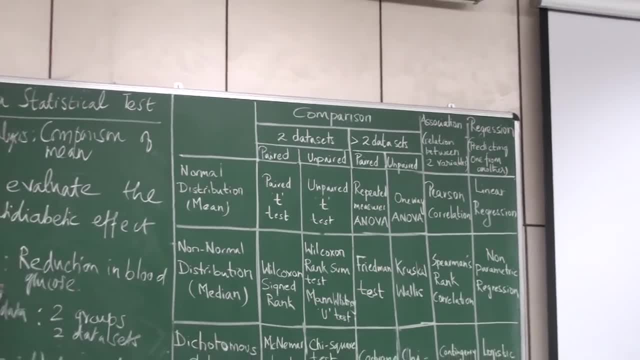 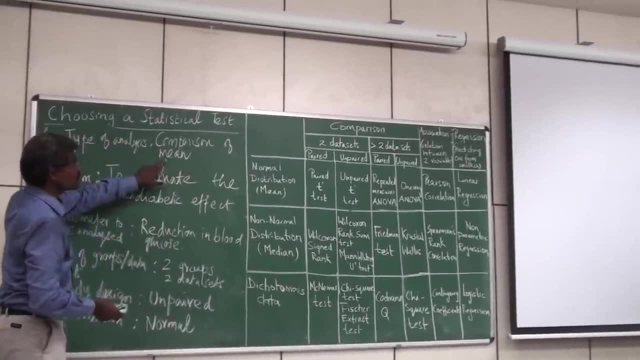 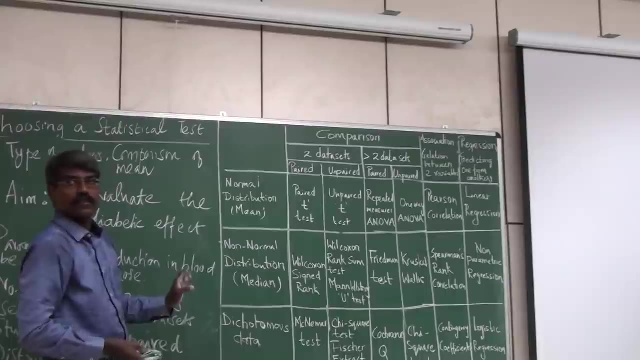 row first. now let's take this example. now, what is our data type? distribution is normal distribution. so I'm what we want to do: comparison of mean, isn't it now now? now look at you and tell me whether we have fixed row one or row two or row three. it's. 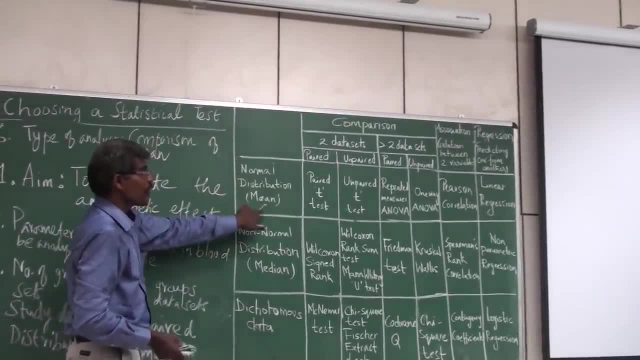 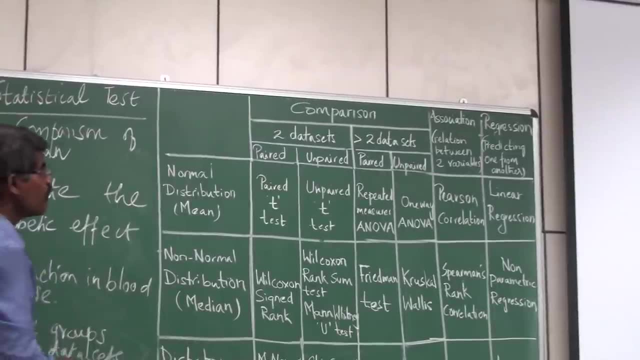 row one, isn't it? because this is normal distribution, which is summarized as mean. so we have fixed row one for this example. now let us fix the column column. let's see it come back now. what do you want to do? what is the type of analysis I want to? 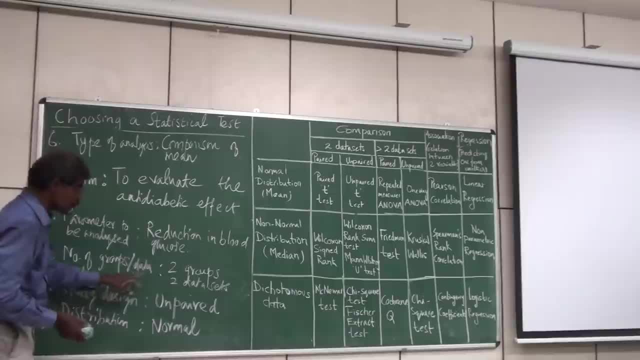 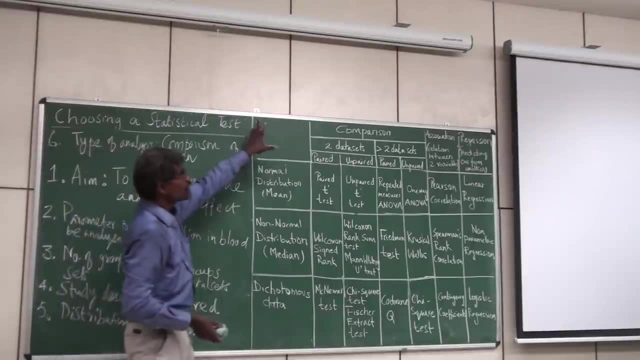 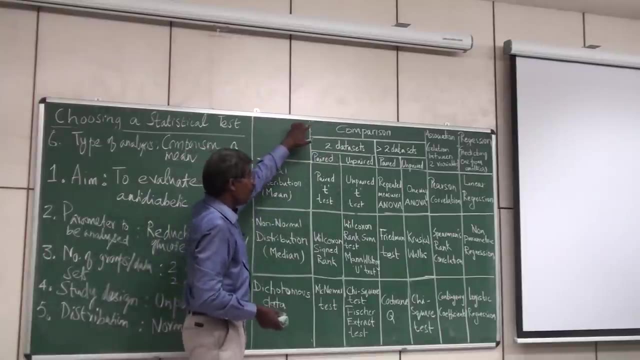 comparison of means. now let me see here how many groups I have. I have two groups, two data sets I have and my design is unpair. now let me fix which bra or column it comes through. it comes to comparison. is it it? because it's not, it's not regression. it's not regression now, the comparison of what two data sets. 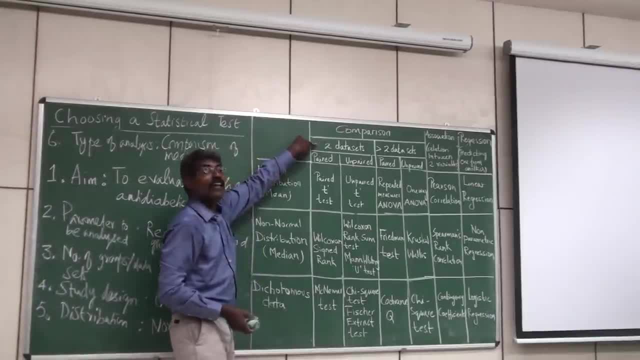 so I have a person of two data sets. now let's go again. what is the beside? it is matrix. we have to take the overall about everything. that side base reaction is: 嘛 did the company which got kind of acted out now letting activity out of it not? 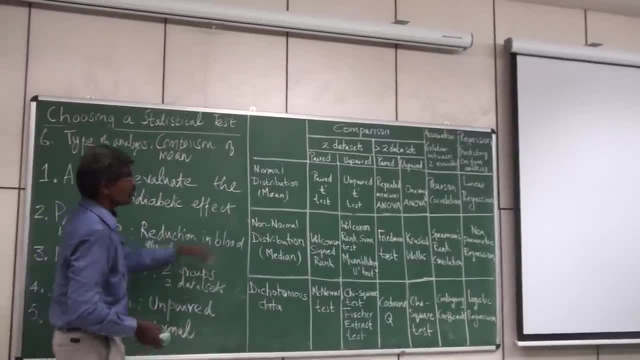 now. then I have to compare with the binary vector which will have the Messiah use from group same time with our Hierophant. this is why I've staff and system from comparisonquinn decide. it's unpacked, so comparison of two data sets and unpacked so I have. 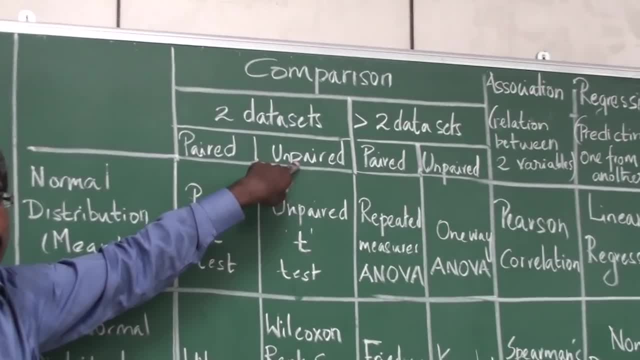 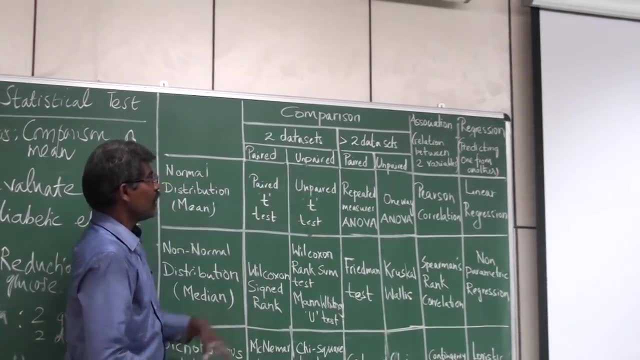 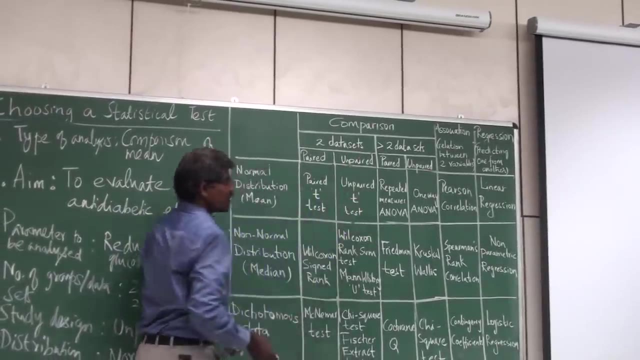 fixed. now which column I belong to. for this particular scenario, I belong to row one and among the two data sets I belong to unpack. now draw an imaginary line connecting the row you fixed on the column you fixed. you end up in the test called as unpacked t-test. so for this particular scenario, the test to be used, 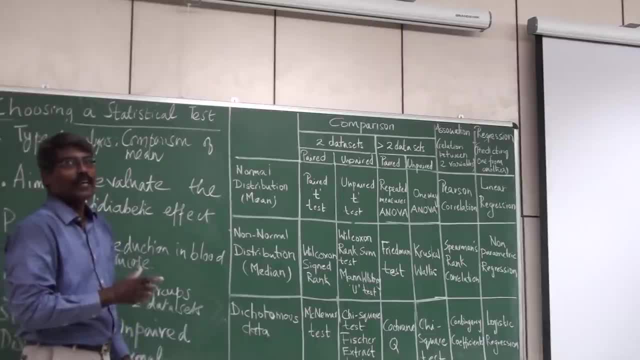 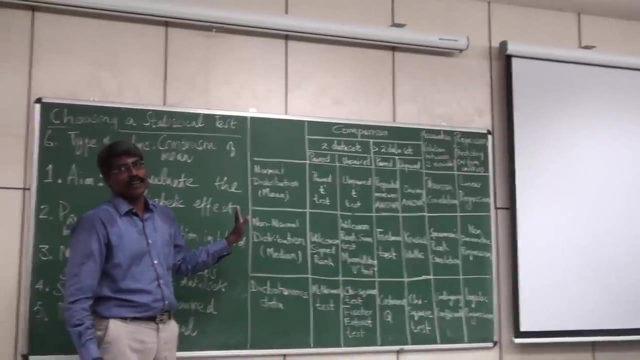 is unpacked t-test. are we clear? so if you follow all these six steps properly and use this table for any type of scenario, you can very confidently find out, and very easily find out, which statistical test you should use for analysis of data. so, to summarize, there are five factors which are which we need. 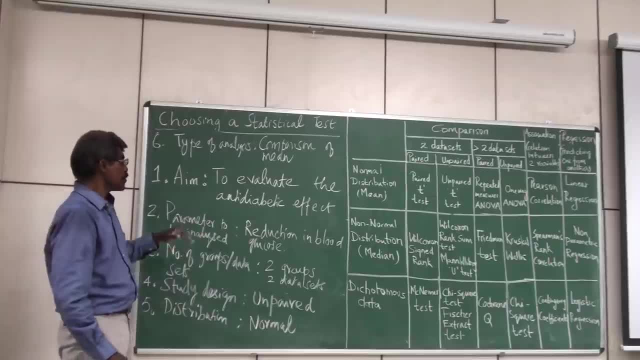 to know, to select which statistical test we want to use. it is, what type of variable we have and what type of variable we have, what type of analysis we want to do, how many groups and how many data sets we have. what is the type of study design in statistical means? it's paired or unpacked. 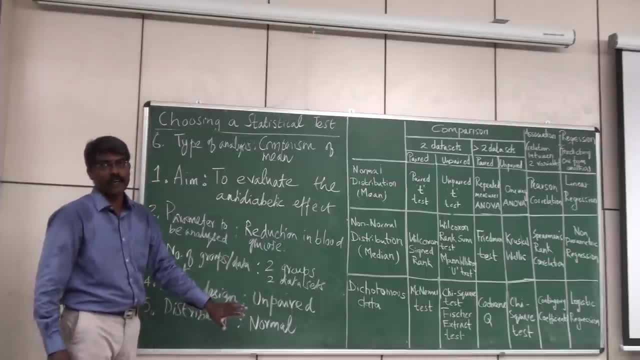 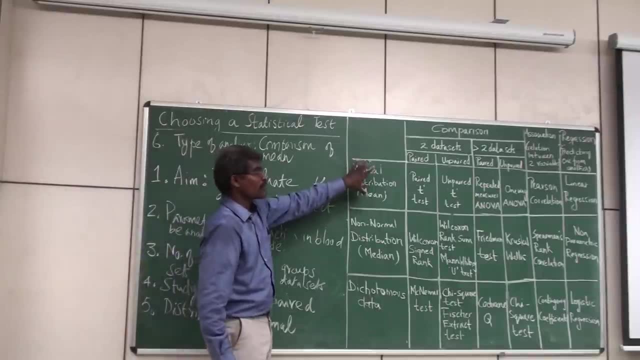 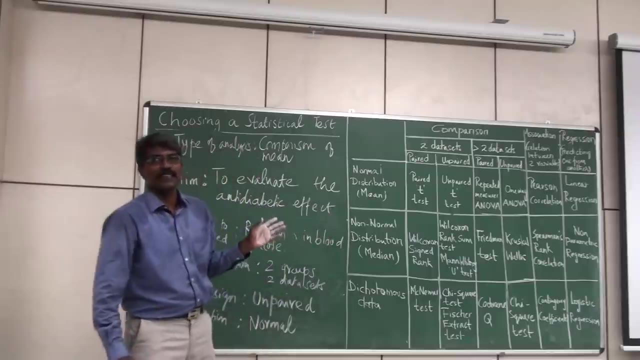 and what type of distribution of data are we dealing with? once we have fixed these five things, go stepwise, write these all these things. then, with the help of table, we need to fix the row and the way that we need to fix the column, draw imaginary line and where does it meet? that particular test is the 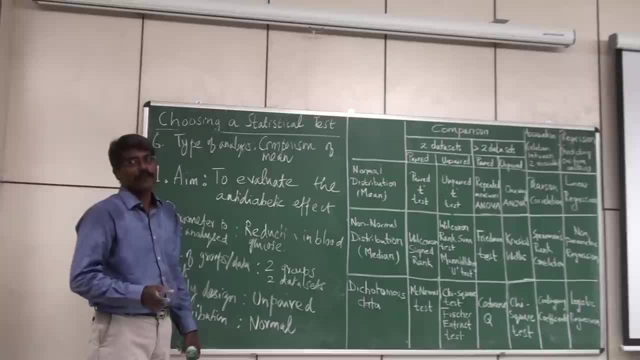 statistical test which you have to use for the analysis of the data set. so this is the test which we want to do. Ok, clear. so this is what we are asking. so for analysis of data, I will repeat that, for this particular study, you might have five or ten variables which you want to. 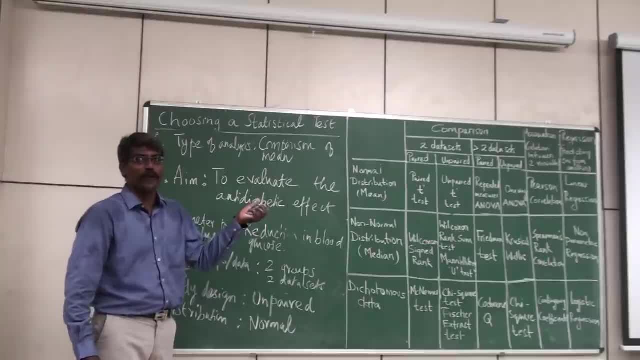 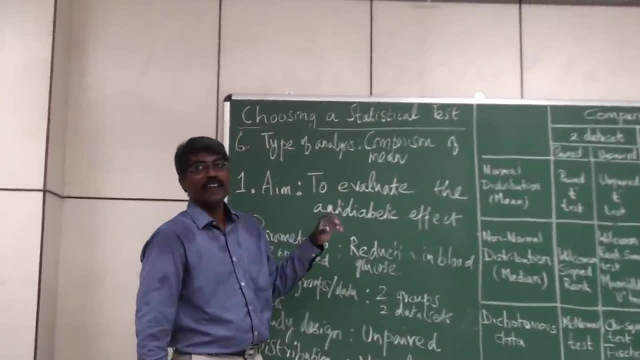 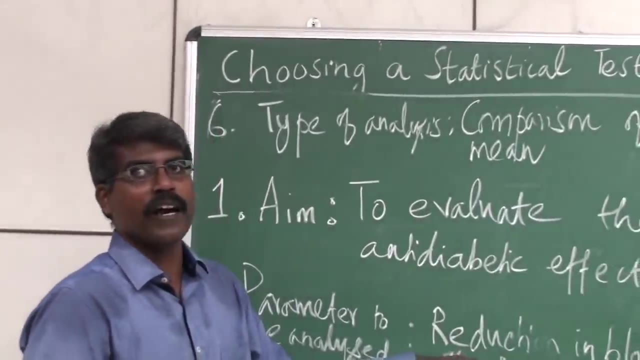 analyze. so for each variable you need to find the particular stress. say, for example, here: if it is blood glucose it has come to unpaired. test the same, if I want to find out if my parameter is number of people on the present day, the proportion of people having adverse effect, then the 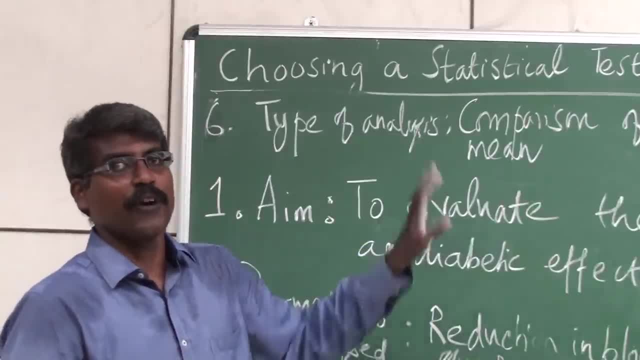 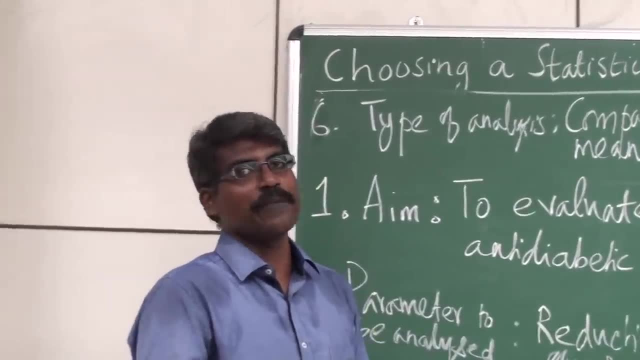 variable completely changes, it will be a totally different test. so for each variable it will always change and you need to look into that. so that's all. if you have any doubts, please get back to us. thank you very much.